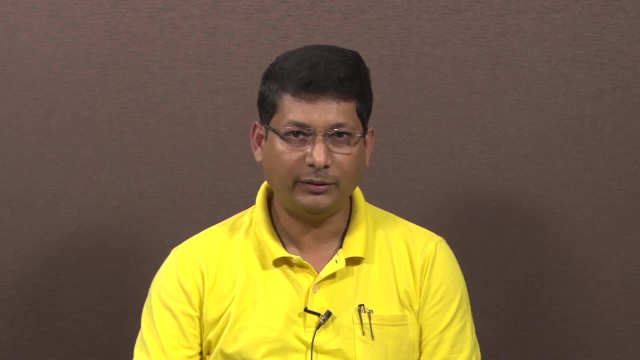 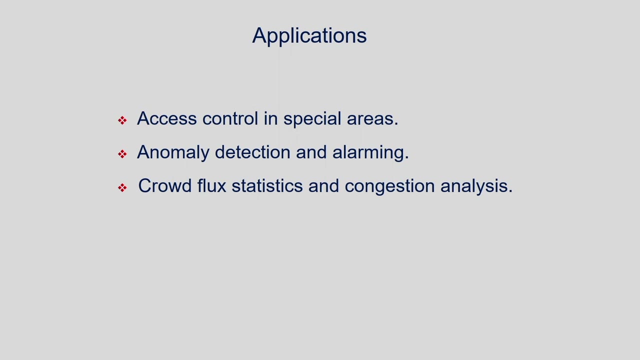 what are the important applications of a video surveillance system? So some of the important applications like access control in spatial areas, like in the airport, railway stations, maybe in the tunnels. So this is one important application, that is, the access control in spatial areas, anomaly detection and alarming. 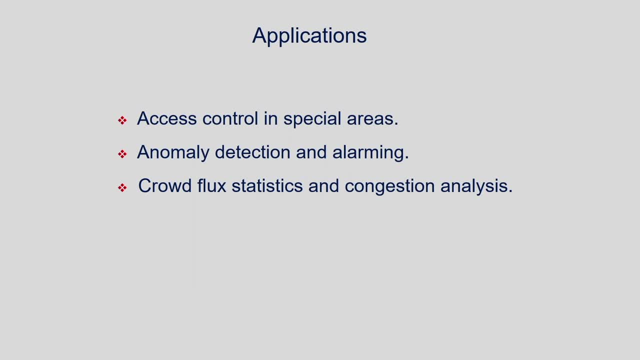 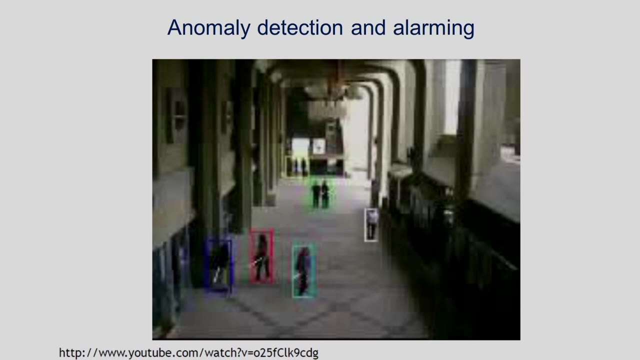 and another one is the cloud flux statistics and congestion analysis. So these are some applications of an automated video surveillance system. So in the figure you can see I have shown one example: the anomaly detection and alarming. So here I am considering you can see the tracking that is. 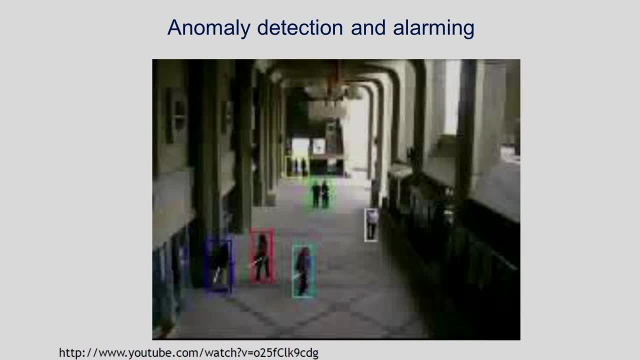 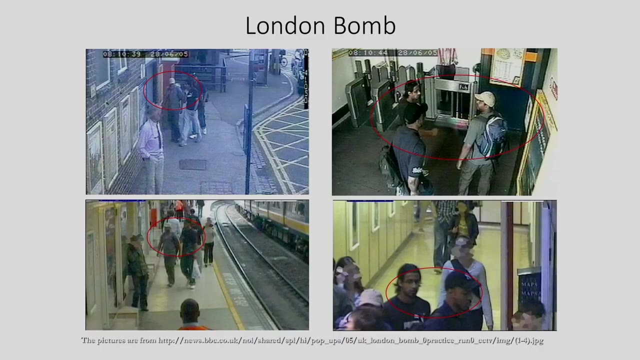 people tracking and from this I want to detect anomalies and accordingly we can give some alarms based on the anomalies. So this is anomaly detection and alarming, And here I have shown one practical example, that is the London boom attack. Here in the figure you can see I have shown some. 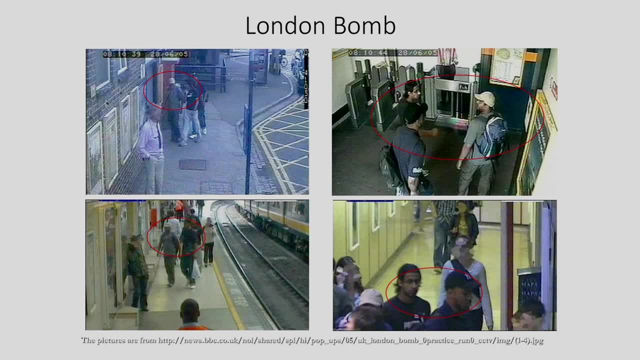 of the frames of the CCTV video sequence and in this case you can see the terrorist were detected by CCTV, So this is related to London boom attack. So I have taken the pictures from this website and this is one application. that is the anomaly detection. Next, also, I have shown some 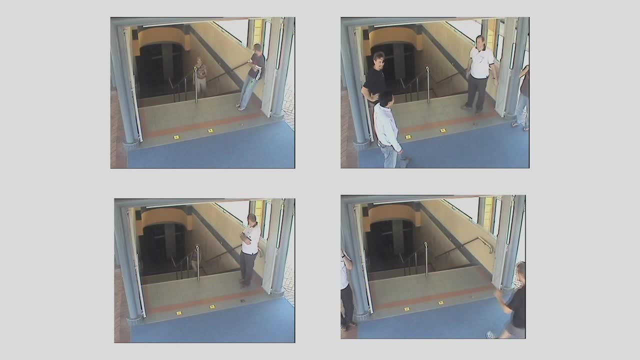 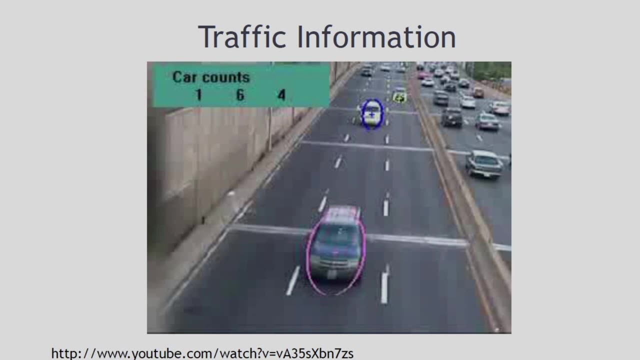 frames of a video sequence that is from the CCTV, and this is nothing but the anomaly detection. And another application is the traffic information. So I can track cars, I can track vehicles and accordingly I can get the traffic information. So this is also one important application. But 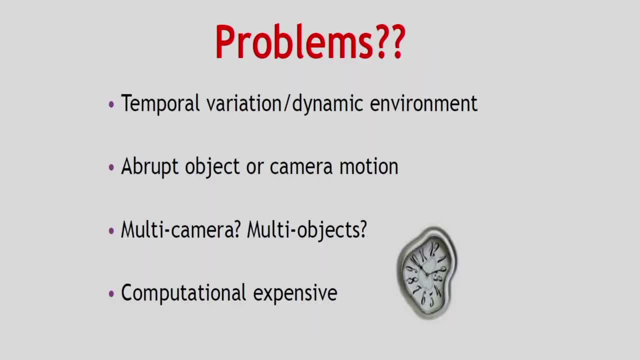 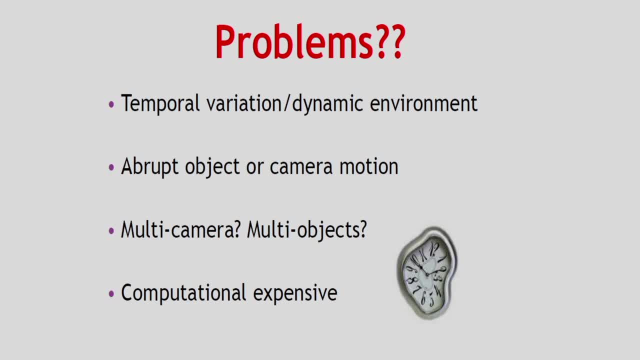 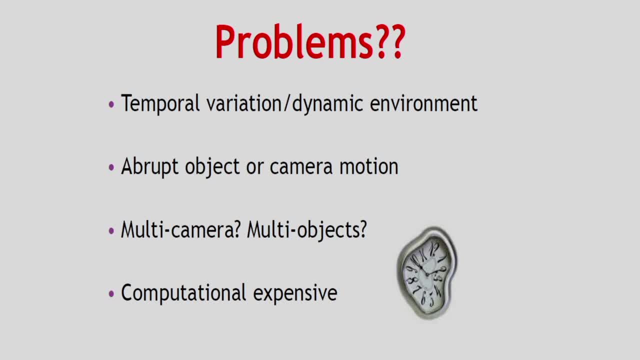 then in this case we have to consider the spatio-temporal variations, as I mentioned in the gesture recognition. In gesture recognition also we have to consider the spatio-temporal variation, In this case also for human activity recognition or maybe the human action recognition we have. 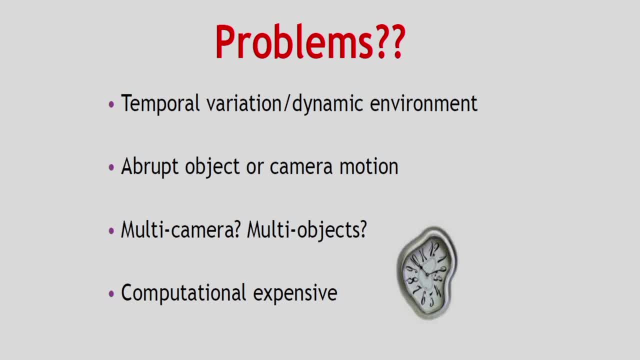 to consider spatio-temporal variations And also whenever I want to detect a person or maybe a particular object, we have to do the segmentation, the segmentation of the foreground from the background. But the problem is the background may be cluttered background or maybe the illumination may changes. 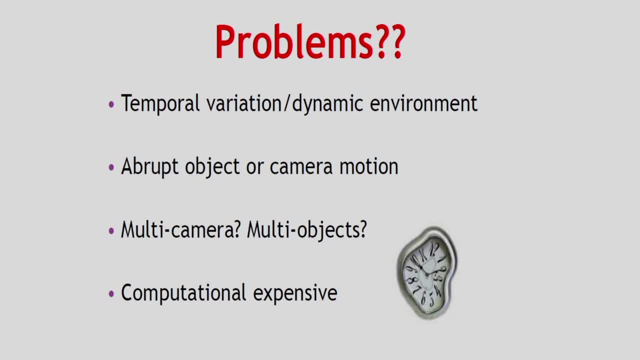 or maybe the background may be the dynamic background, Then in this case it is very difficult to do the background subtraction. For all these conditions, particularly the illumination variations- Cluttered background, dynamic background- it is very difficult to do the segmentation, The segmentation of the foreground objects from the background. 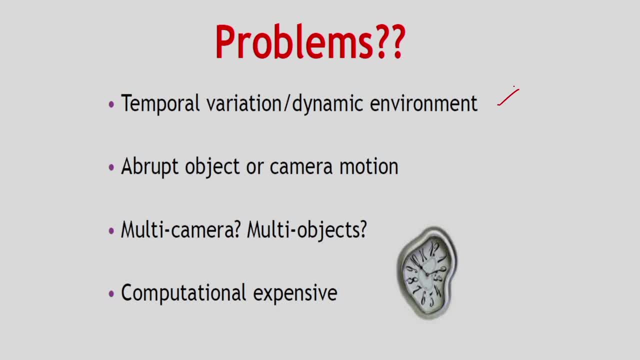 So that is the dynamic environment and also the temporal variation. The next point is the abrupt object or the camera motion. So there may be abrupt object or the camera motions. Then in this case also we have to do the tracking, We have to do the background subtraction. 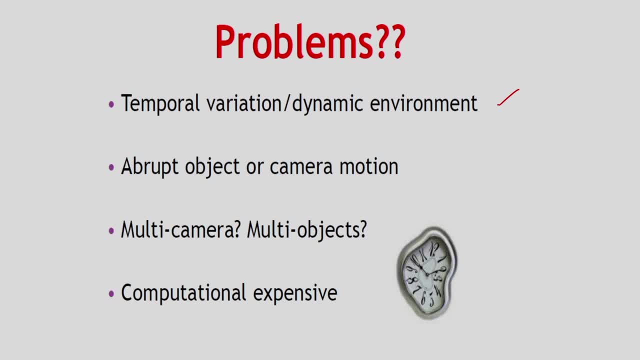 So all these things we have to do, But we have to consider these cases, that is, the abrupt object or the camera motion. And also we can employ multiple cameras for a video surveillance system. So for multiple cameras the field of view will increase as compared to single camera. 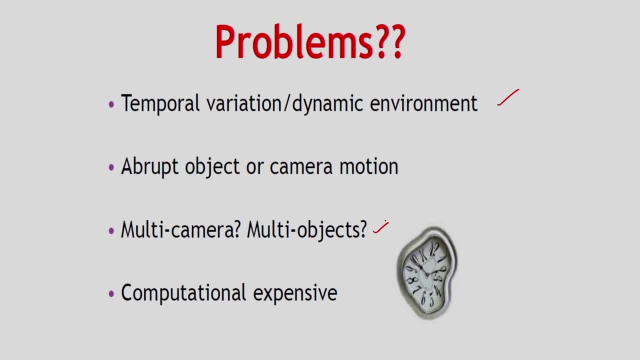 But the problem is I have to find the correspondence between all these cameras, the multiple cameras. So that is one research problem. So how to find the correspondence between all these cameras available in the video surveillance system? Also, we need all the outputs in the real time. 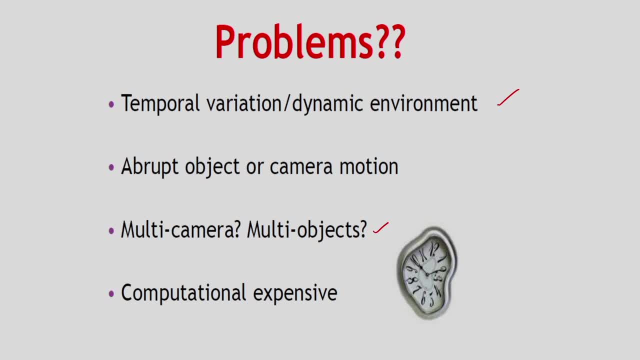 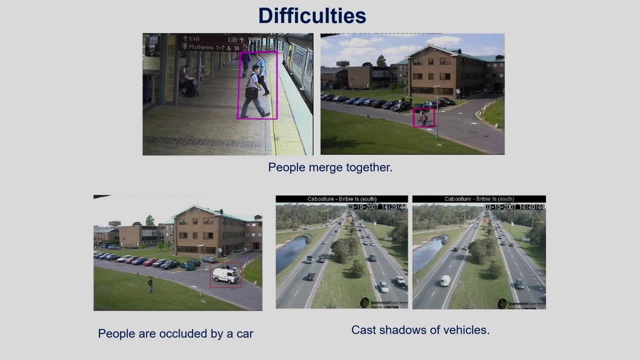 So that is why one important issue is the computational complexity of the algorithm. So these are the main problems for an automated video surveillance system. So again, I am showing some of the difficulties. In this case I am showing the concept of the tracking, But 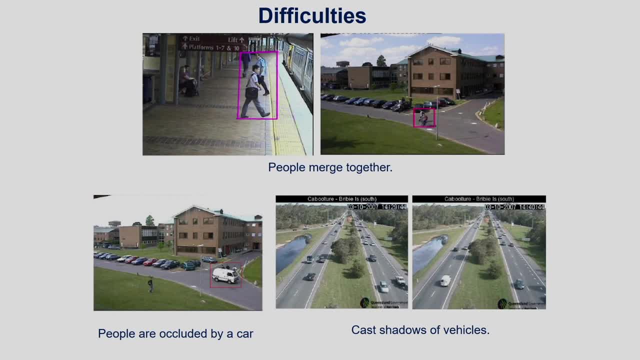 In the image you can see the people merge together. That means there may be some occlusion And because of this occlusion it is very difficult to track. So here you can see the people merge together. In this case also, the people merge together. 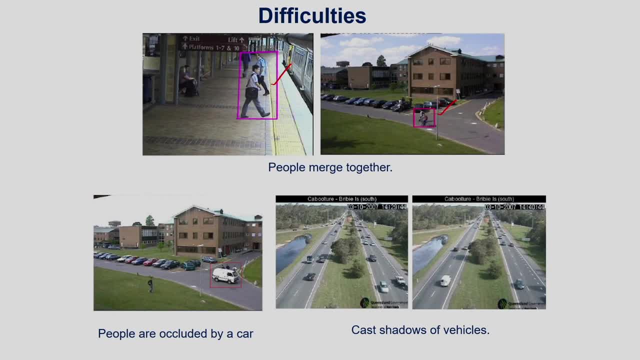 In this case also we have to do the tracking. But it is a difficult situation, So in this case also we have to do the tracking. Next one is the people are occluded by a car, And that is also another example of the occlusion. 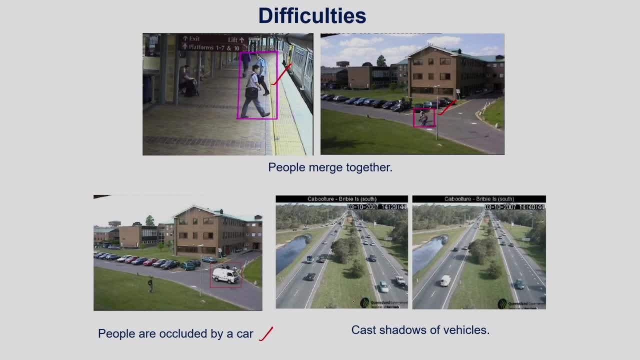 So for a particular time maybe people are occluded by a car, Then also we have to do the tracking. So this is one difficulty And also, if I consider the tracking of vehicles, then the problem will be the shadow. Even for the tracking of people the problem may be the shadow. 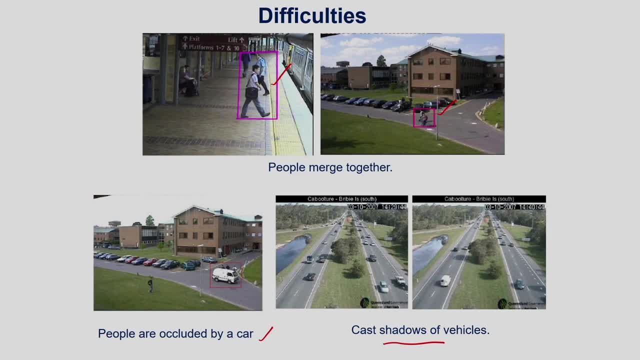 So the cast shadow, that means the shadow of the vehicle we have to consider. So vehicle will be moving at a particular speed And its shadow will be also moving. So in this case we have to do the segmentation, The segmentation of the vehicles from the background. 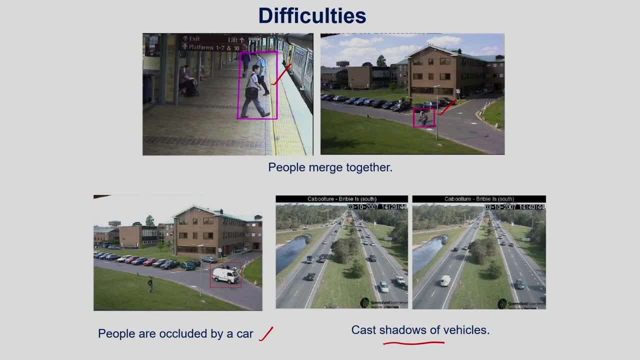 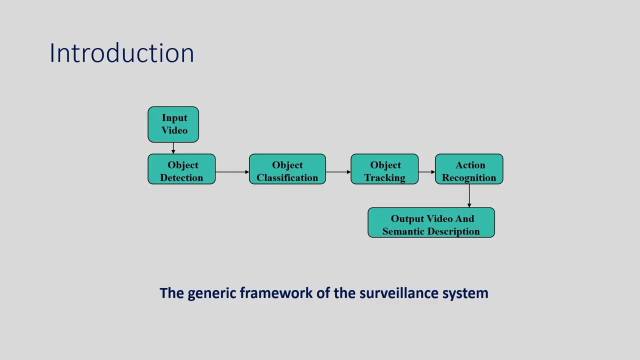 And after this we have to do the tracking. So the tracking in presence of shadow is a big difficulty. So we have to do this, We have to remove the shadow, And that is also another research problem in video surveillance. So let us consider one generic framework of a video surveillance system. 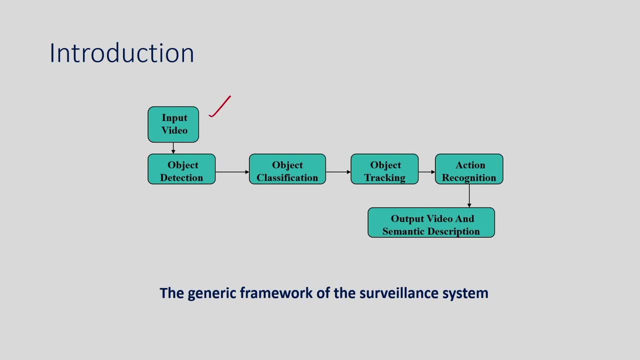 So input is the video surveillance. After this we have to detect the objects present in an image And after this we can employ some machine learning algorithms, The pattern classification algorithms for object classification. After this we can do the tracking, The tracking of the objects. 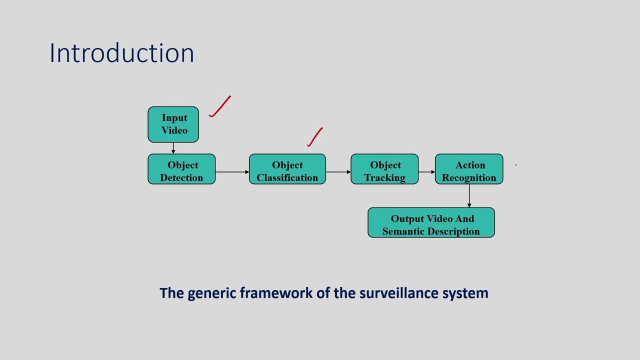 And also we can employ this one, That is the action recognition we can do. That is the activity recognition. Suppose the people are walking or people are standing like this. So for this we can recognise different actions. That is similar to the gait recognition. gait means the walking style. 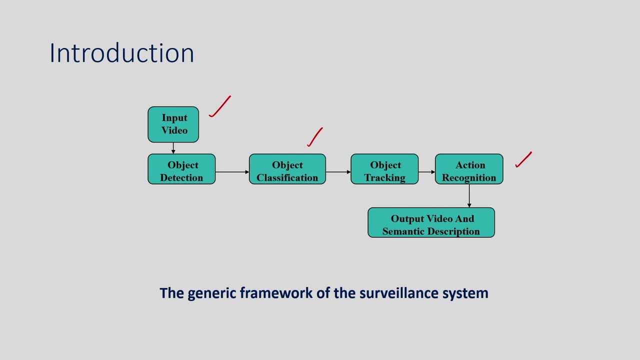 So that is we can do, that is action, recognition, And output is the output video and the semantic description. So I will be getting the semantic description of the input video. So this is a generic framework of a video surveillance system And you can see what is the difference between the object detection and the object cartoon. 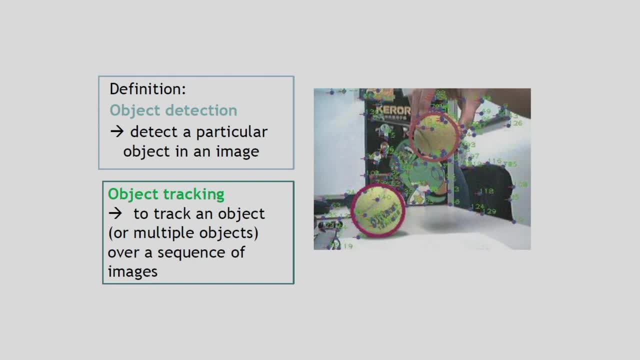 tracking. So object detection means detect a particular object in an image. So here you can see: I am detecting these objects and that is nothing but the object detection. But what is the object tracking? To track an object, or maybe the multiple objects over a sequence of images? 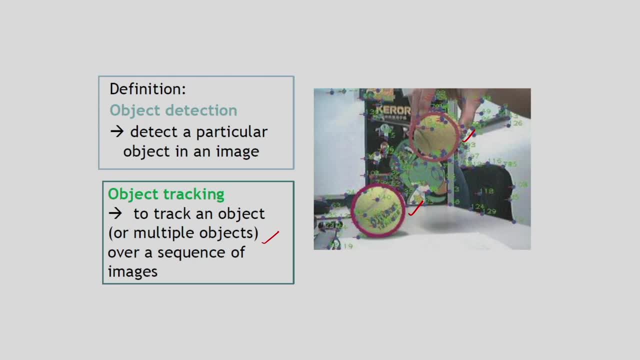 that means the sequence of images, means the frames of a video. So in this case I have to find the correspondence between the frames of a video. that is, to track an object, maybe a single object or maybe the multiple objects, over a sequence of frames of a video. that is the object tracking. 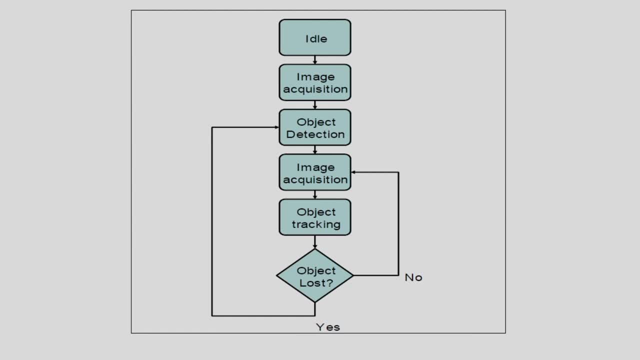 And how to detect the object that. I am showing one simple flowchart here. So suppose the object is stationary. after this we are considering the image equation. after this we can detect object. So object detection algorithms are available. after this, again the image equation from the video that 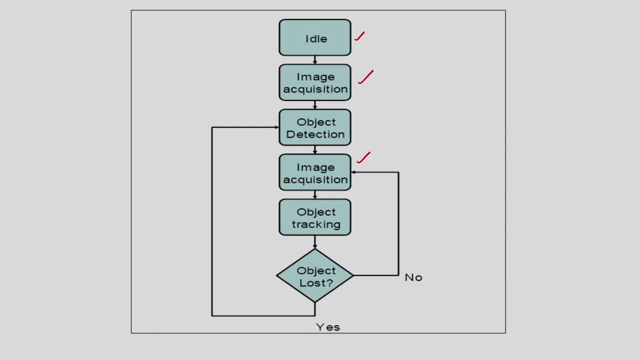 is the frames I am collecting or the frames I am taking from the video. and after this again I am doing the object tracking and suppose the object is lost in a particular frame. then again we have to detect the objects and if the object is not lost then we can continue the tracking. 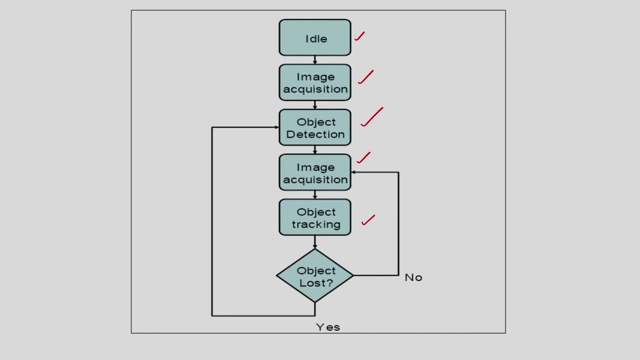 So you can see. first I have to detect the object present in an image or present in a video. after this we have to do the tracking. in some of the frames the objects may get lost. then, in this case again, we have to acquire the frames of the video and we can detect the object. and after this, 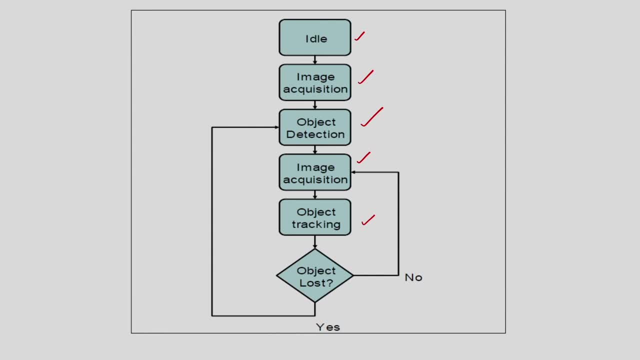 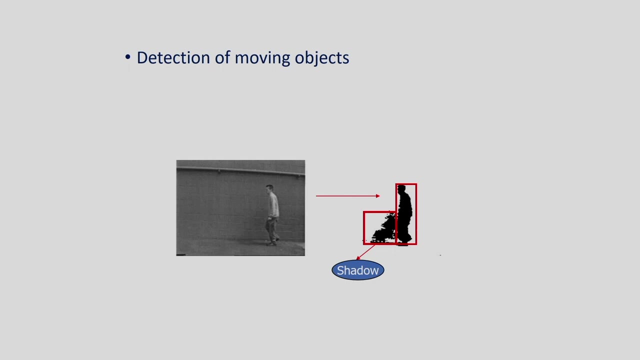 we can continue the tracking like this we can do, but the object, if it is not lost, then we can continue tracking. So this is a simple flowchart to detect objects and also do the tracking. So here you can see I am showing one example: detection of the moving objects. and this person is moving and we have to. 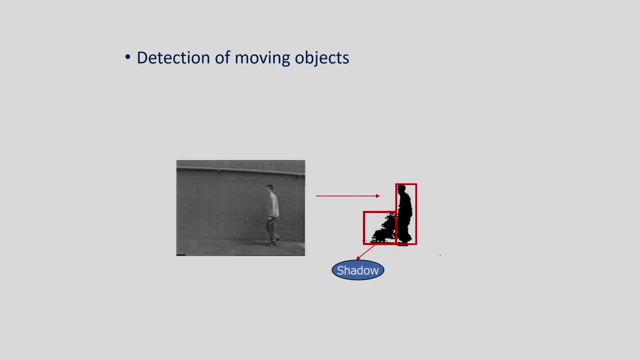 detect the moving objects based on some algorithms, but the problem is the shadow, that is the cast shadow we have to remove. the person is moving and his shadow is also moving, So that is why the problem is detecting the moving objects. So that is why we have to develop some algorithms so that 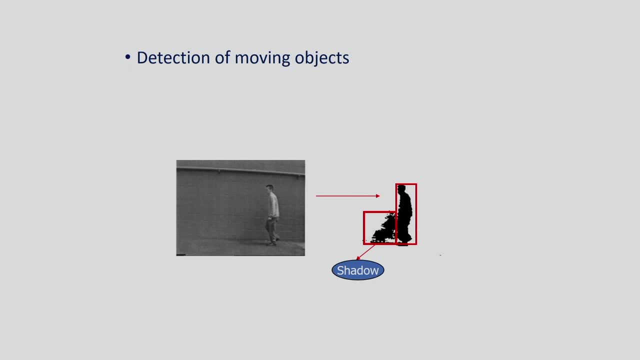 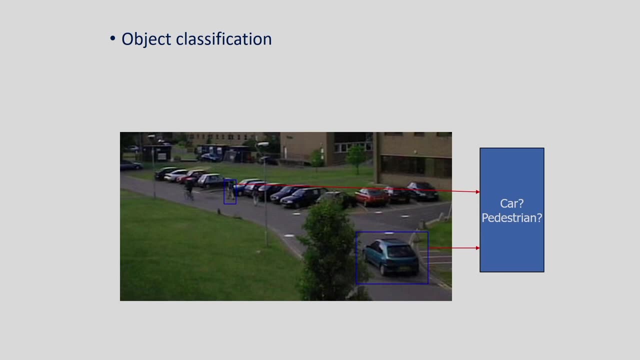 we can remove the shadow. that is the problem of detecting the moving objects in presence of shadow. after this, object classification, So we can consider the classification of objects present in an image or maybe the video. So here you can see, we are classifying the objects. 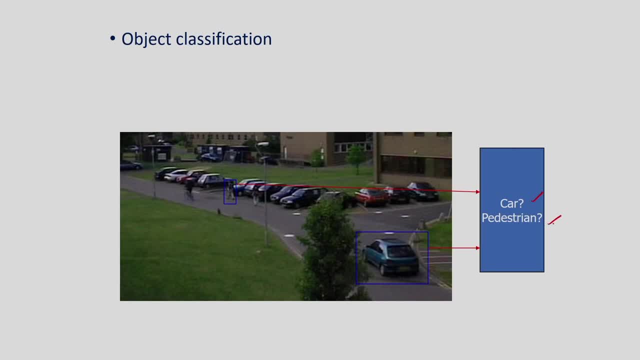 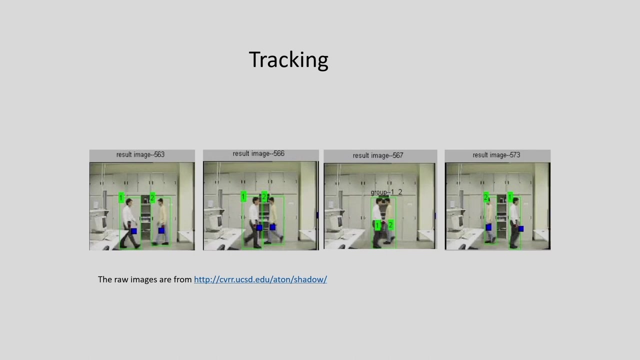 the car, the pedestrians, like this. we can do the classification based on some algorithms. that is also very important. So we can employ some machine learning algorithms for object classification and the tracking. already I have explained: it is nothing but finding the correspondence between the frames of a video. In this case, I have shown some of the frames of a. 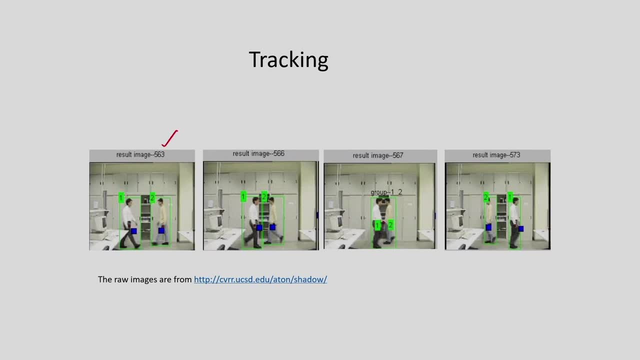 video. So here you can see the 563, that is, the frame number 566, 567. like this: these are the frames and you can see the person 1 is moving and person 2 is also moving and there may be occlusion in this. 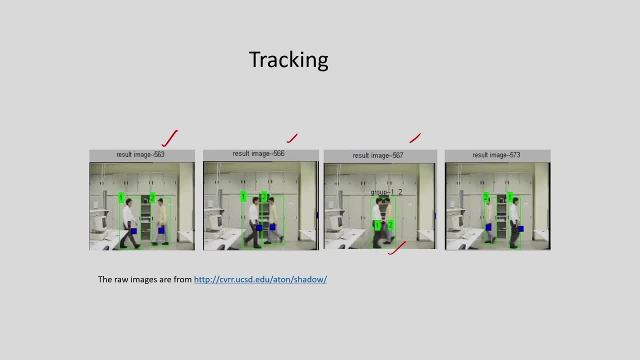 case. you can see in the image 567, there is a occlusion and in presence of the occlusion also we have to track the person, the person 1 and person 2- and you can see the output of this, the tracking algorithm. So we can track person 1 and the person 2 in this video. So 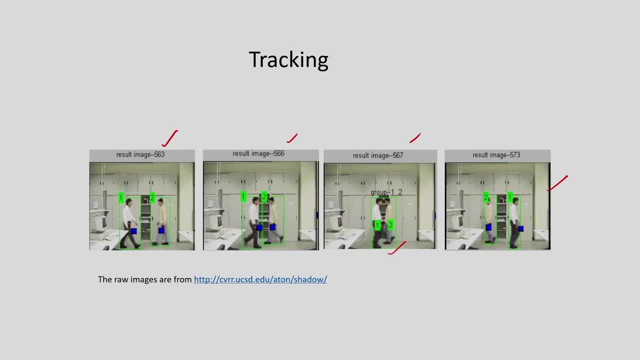 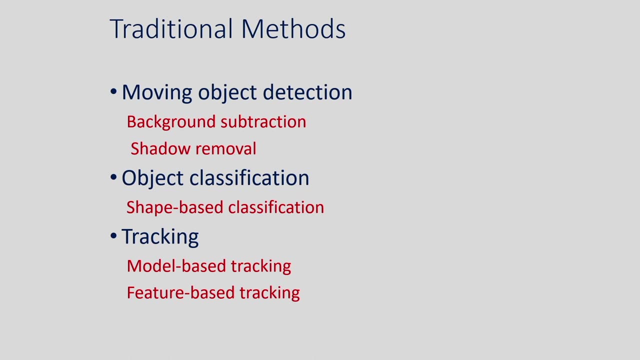 tracking means the finding, the correspondence between the frames of a video. So some of the traditional methods for all these activities: for moving object detection we can employ the background subtraction algorithm and also we have to remove the shadow, that is the shadow removal algorithm we have to employ For object classification. simply we can employ the 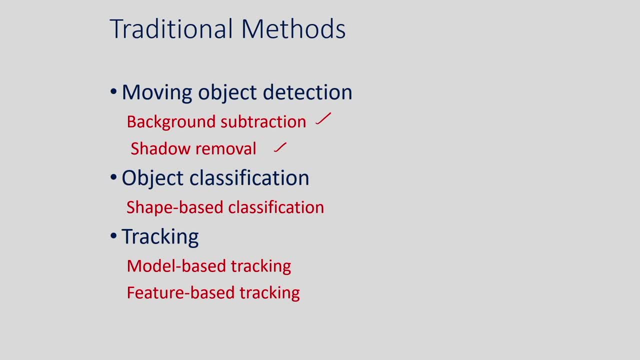 shape information, that is, the shape based classification we can do, and for tracking of the objects we can employ the model based tracking and also the feature based tracking. In case of the model based tracking, we can consider the model of the object, maybe the geometrical model we can consider, and based on this model we can do the tracking. 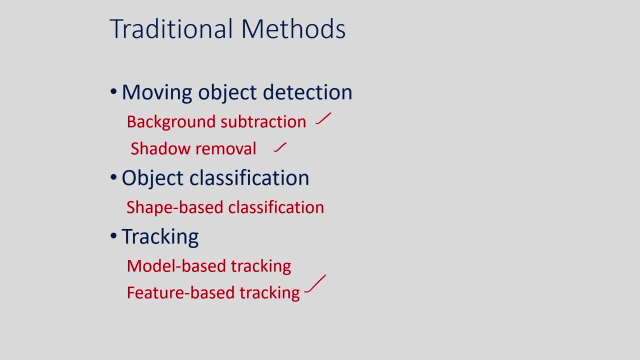 In case of the fissure based tracking, we can consider some of the fissures, maybe the color fissure, maybe the texture. So all these features we can consider and based on these features we can do the tracking. So these are the traditional methods employed in the video surveillance system. 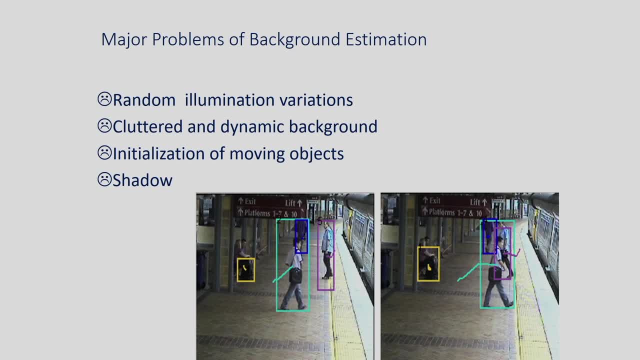 Then the major problems of the background estimation. so one is the random illumination variations that we need to consider. So illumination is not uniform. So if if there is a random illumination variation, then the problem of the background subtraction, the background estimation and the background may be cluttered, and also the dynamic background. 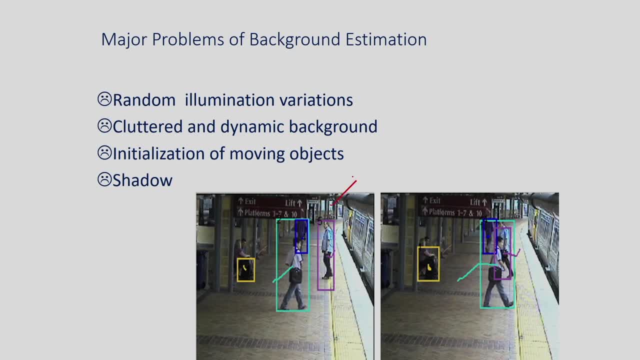 So in this image you can see the background is very cluttered and one train is moving. that means the background is dynamic And we want to track these persons. ah, you can see I am doing the tracking in presence of the moving background and the cluttered background and also the illumination is not. 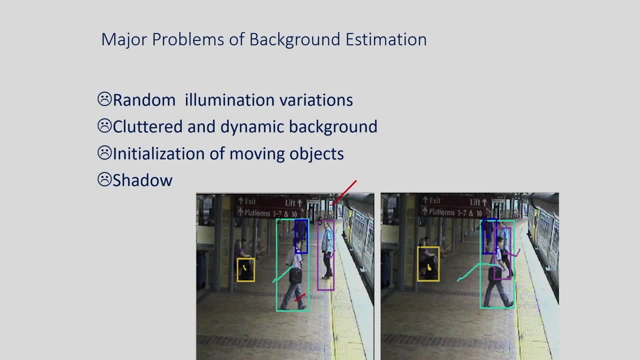 constant, not uniform. Random illumination variations are ah available in this ah images, in the video. And also we have to do the initialization of the moving objects In this video or in this images or in this project, In this frames of the video. you can see, ah, you can see ah, we have the moving objects. 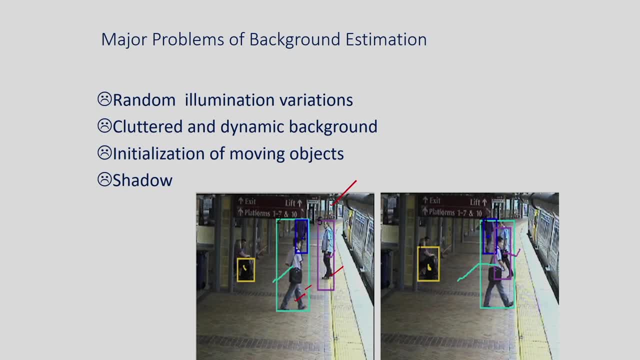 ah, this person is moving. this person is moving, So we have the moving objects and also some persons. they are sitting here, that means they are stationary, So we have to initialize the moving objects And also, as I explained earlier, so we have to consider the shadow problem. 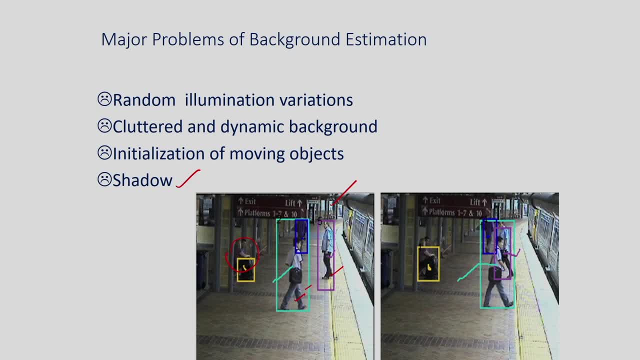 And one difficult problem is the removal of the cast shadow, Because the shadow is also moving and the person is also moving. So, based on the motion information, I cannot do the separation between the moving objects and the shadow. So we have to employ some algorithms so that we can remove the cast shadow. 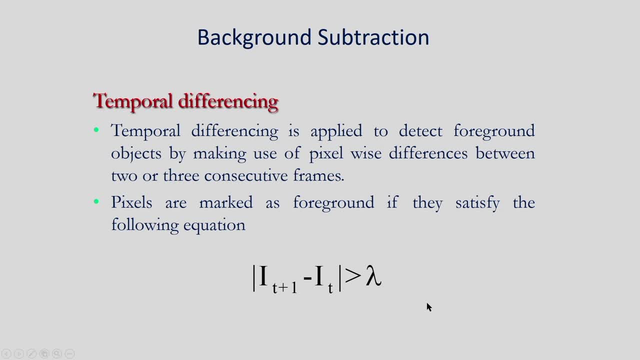 Now I will discuss the concept of the background subtraction. So one ah very old algorithm is the temporal differencing. So this algorithm I can apply to detect, ah, to detect foreground objects by making use of pixel wise differences Between 2 or 3 consecutive frames of the video. that means I have to, ah, find the differences. 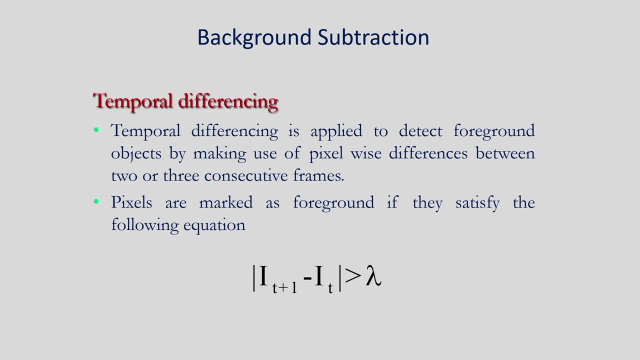 between 2 or 3 consecutive frames And the pixels are mark as foreground if they satisfy the following equation: Suppose, if I consider a particular pixel, the pixel at the time t plus 1, is this: it plus 1 minus it, that is a pixel, that pixel at the time t. 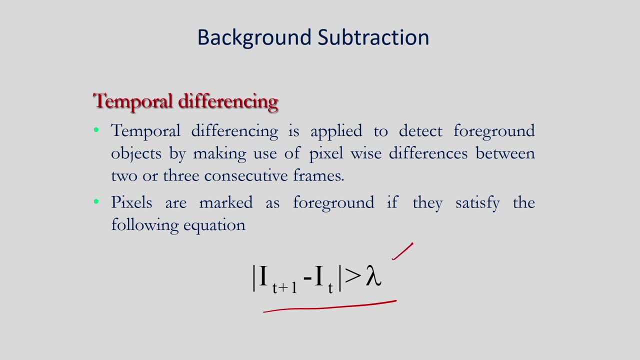 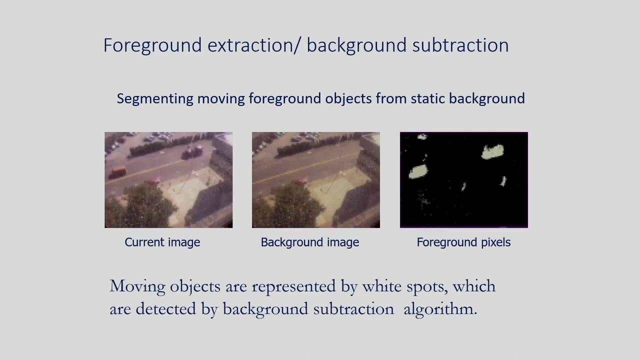 difference between this is greater than a particular threshold, then we can consider that pixel as a foreground pixel. otherwise it is a background pixel. Like this we can determine the moving pixels In this case. I am showing one example of foreground extraction, that is the background subtraction. 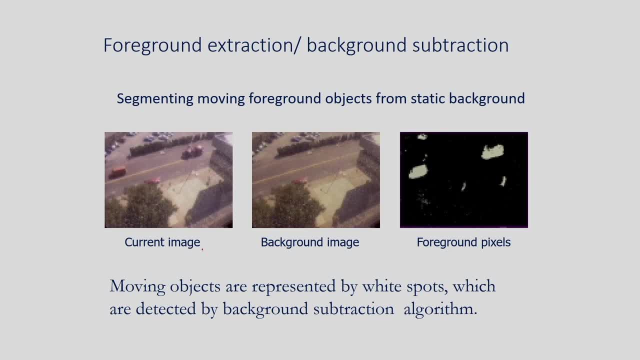 that is nothing but the sense detection algorithm. So this is the current image and I am considering the background image. If I subtract the background image from the current image, I will be getting the foreground pixels. So this is nothing but the background subtraction algorithm. 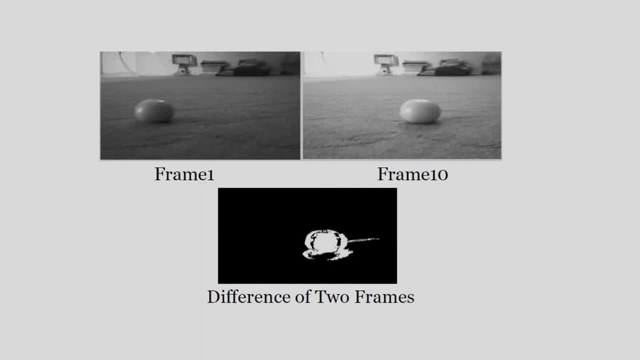 So again I am showing the same thing: the background subtraction algorithm. So this is frame 1, another one is the frame 10.. So if I do the subtraction, then I will be getting the difference of the two frames. that is nothing but the moving objects I can determine. 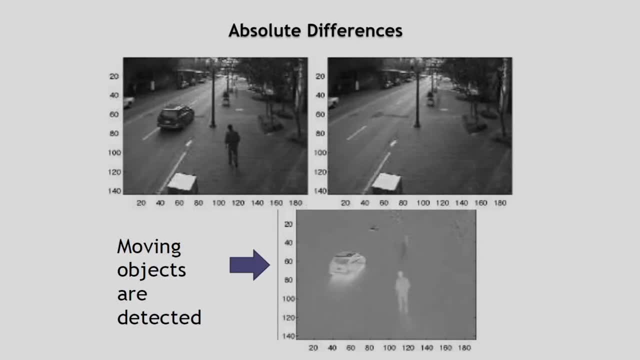 And similarly I am showing one example of the absolute differences. So two frames I am considering, So you can see, in the first frame the moving objects are present, In the second frame the background, that is the nothing but the background. And if I subtract the second image from the first image I will be getting the moving objects. 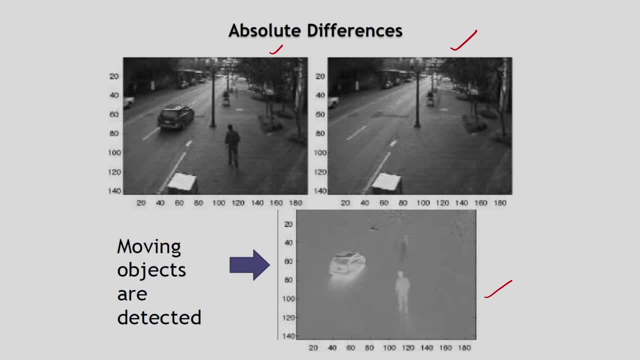 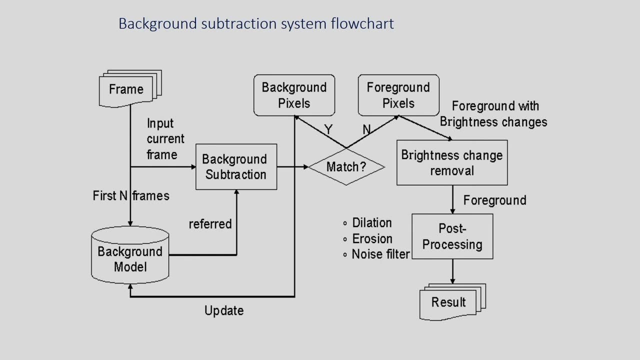 That is, the moving objects will be detected. That is nothing but the absolute differences. So in this example I have shown one algorithm, that is a simple algorithm for background subtraction. So background subtraction system flusher. So suppose I have the input video And I am considering the frames of the video. 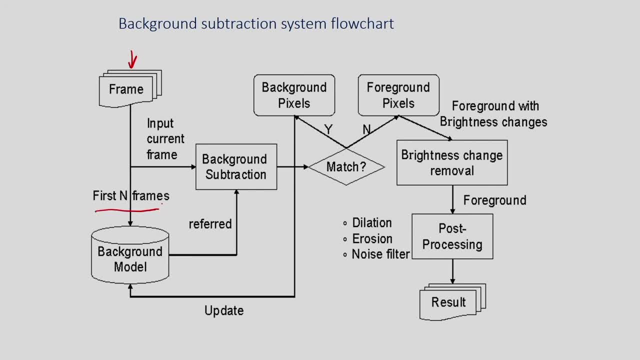 First I am considering the n frames. the first n number of frames I am considering And based on this I am determining the background model. So the background model is determined from the first n number of frames. After this, suppose one input frame is coming, that is, the input current frame. 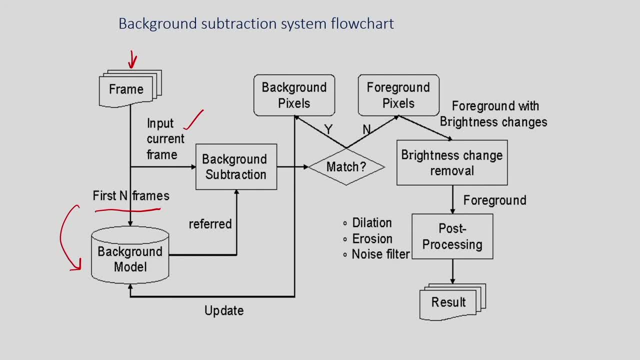 And I can employ the background subtraction algorithm. So you can see, I have the background input, I have the background image here And I have the input current frame. So I can employ the background subtraction algorithm And based on this, I can determine the foreground pixels and the background pixels I can determine. 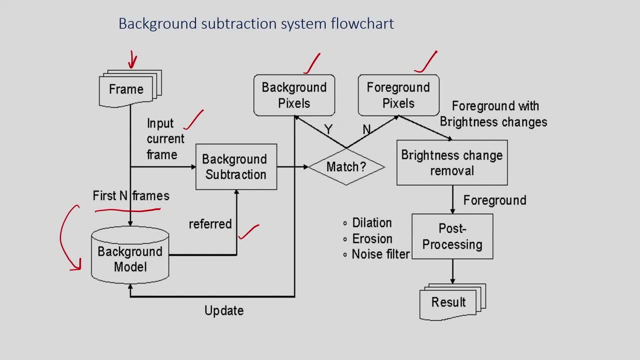 based on the matching And this based on the background pixels, I can update the background model that already I have developed from the first n number of frames. And also I have to consider the brightness sense removal. So there may be sense removal. So there may be sense removal. 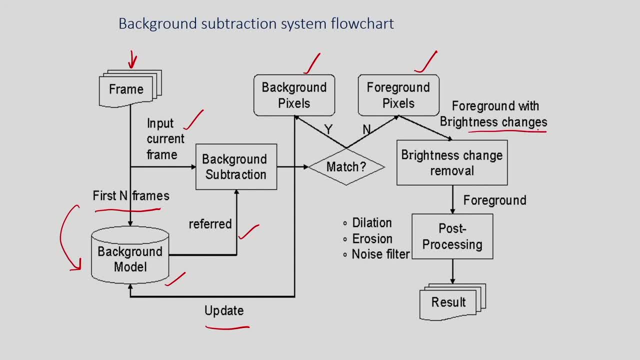 So there may be changes of the brightness. So that also we have to consider, And I will be getting the foreground After this: we have to do some post-processings So maybe we can employ the morphological image processing operations like the dilation erosion. 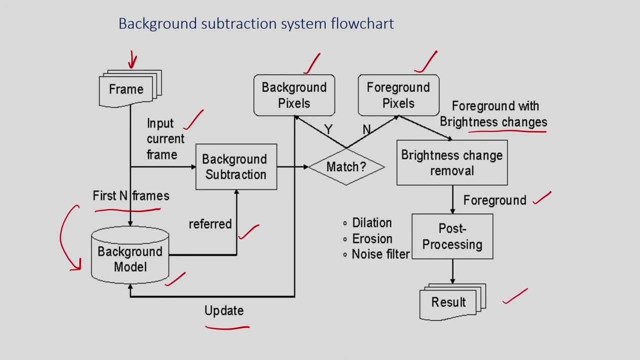 noise filter like this we can employ And ultimately, I will be getting the output that is nothing but the foreground image I will be getting. So I can separate foreground and the background by considering this background subtraction algorithm, And this is also very old technique. 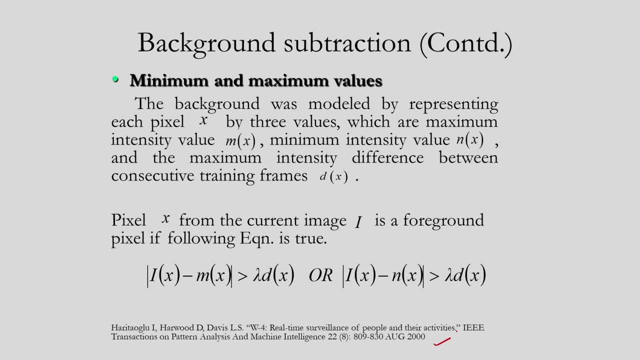 Here it is published here. that is IEEE transaction on pattern analysis and machine intelligence. So, briefly, the concept is like this. So the background is modeled by representing each pixel. The pixel is x by three values. So three values are considered. One is the maximum intensity value, mx. 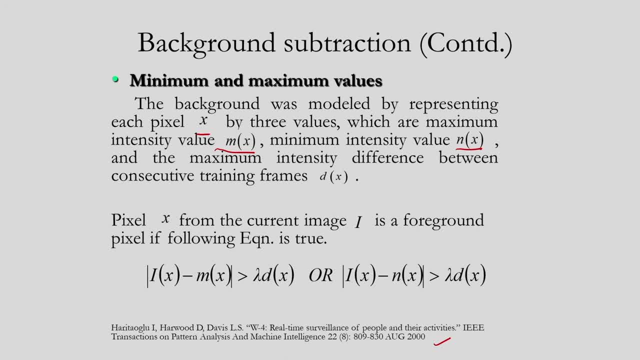 One is the minimum intensity value nx, And the second one is the maximum intensity value nx. And the third one is the maximum intensity value nx And the maximum intensity difference between the two conjugative training frames, That is the dx. So by using these three values, one is the maximum intensity value. 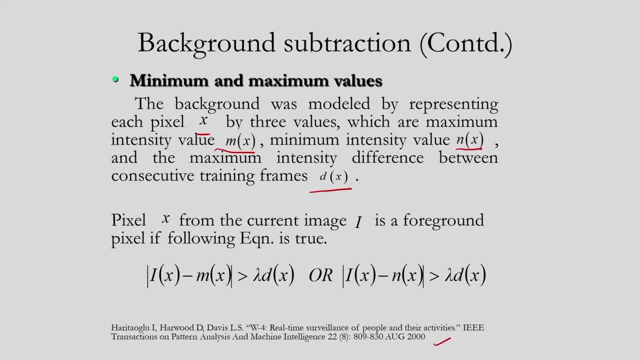 Another one is the minimum intensity value And another one is the maximum intensity difference between conjugative training frames. I can develop the background model. So how to do this? So pixel x from the current image i is considered as a foreground pixel If the following equations or the following equation is true: 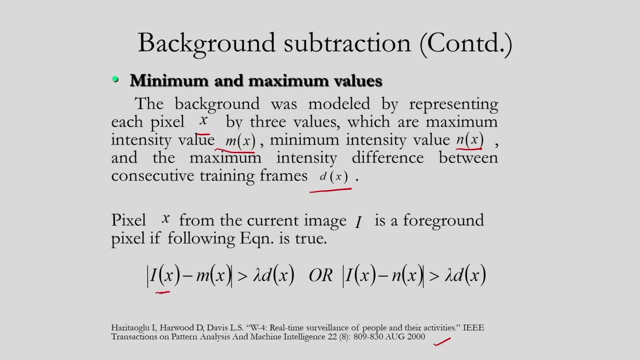 That means ix, that is the current pixel minus mx. What is mx? That is the maximum intensity value. mx is greater than lambda dx. or maybe ix minus nx. Nx is nothing, but the minimum intensity value is greater than lambda dx. So based on this I can determine the foreground pixels. 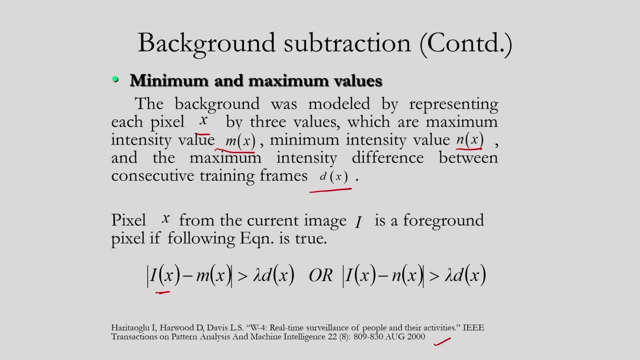 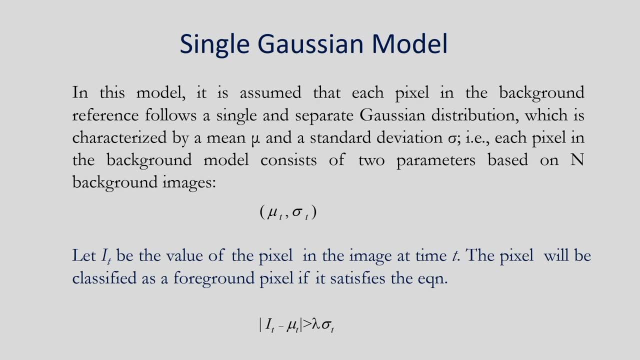 So this is the minimum intensity value And this is also a very popular technique for background estimation, background modeling. So, briefly, this is about the algorithm. So based on this, I can determine the foreground pixels, And this is also a very popular technique for background estimation, background modeling. 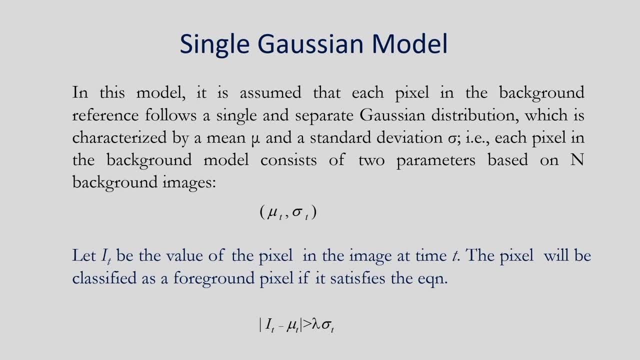 So we can employ single Gaussian model. So in this case what we can consider is pixel in the background. reference follows a single and separate Gaussian distribution. So that means each pixel in the background. So that means for a particular pixel we can consider a Gaussian distribution. 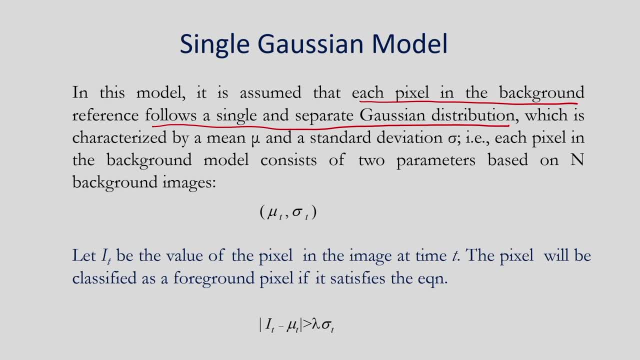 And which is characterised by the mean and the standard deviation. So that means each pixel in the background model consists of 2 parameters based on n number of background images. So we can consider n number of background images. So from n number of background images we can determine the mean. 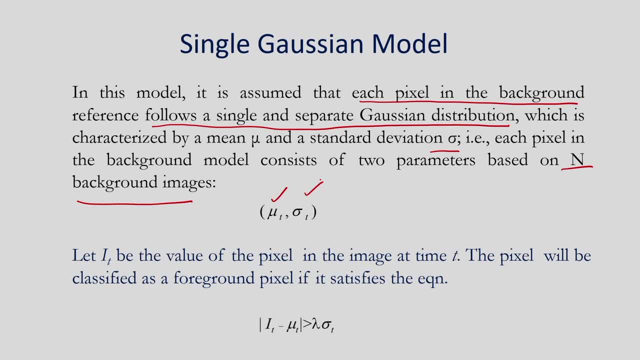 And theって standard deviation that we can determine. And that is nothing but the background model of the image, And suppose i t be the value of the pixels in the image at the time t. so suppose I am considering the pixel at the time t. the pixel will be assigned or may be classified as a. 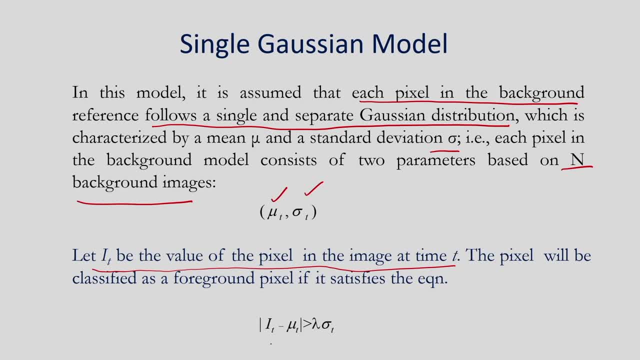 foreground pixel. if it satisfy the following equation, so this equation should be satisfied. So i t means the value of the pixels in the image at time, t minus the mean, is greater than lambda sigma t. if this condition is satisfied, then I can consider that particular. 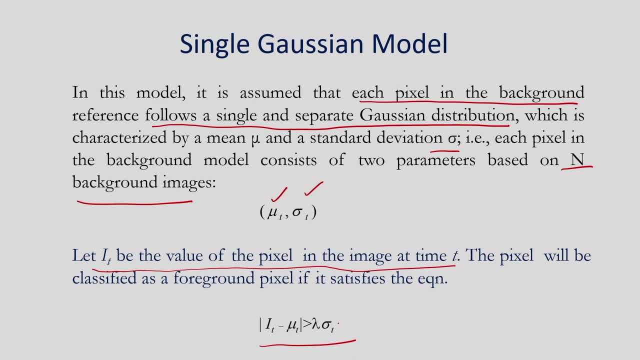 pixel as a foreground pixel. So lambda is a user defined parameter and I am considering the difference between the pixel and the mean that I am considering i t minus mu t. if it is greater than lambda sigma t, Then we can consider that particular pixel as a foreground pixel. 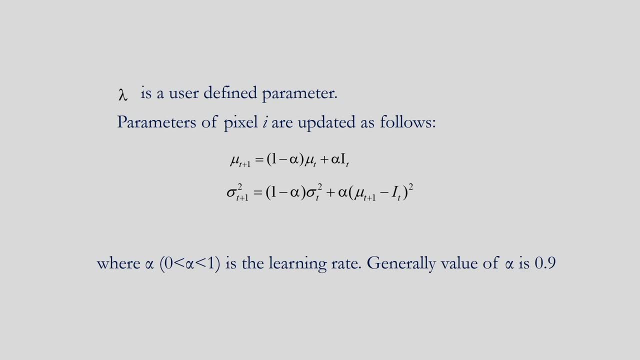 So lambda is a user defined parameter and after this, the parameters of the pixel i should be updated Again. we have to update the parameters corresponding to the pixel i. so the mean is updated like this and also the variance I can update like this. So these are the updating equations and in this case the alpha is a parameter and that. 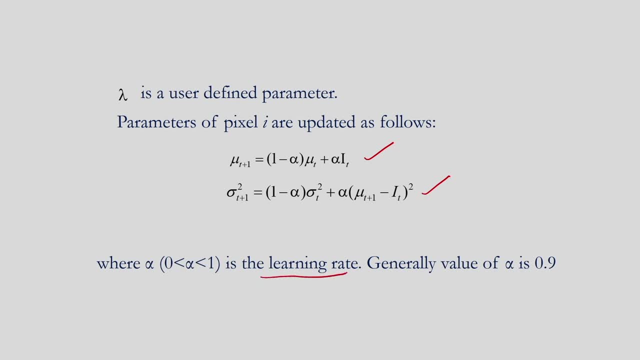 is used for this. And thirdly, I can control the learning rate. So I can control the learning rate based on the value of the parameter alpha, and generally the value of alpha is 0.9.. So this is the concept of the single Gaussian model. 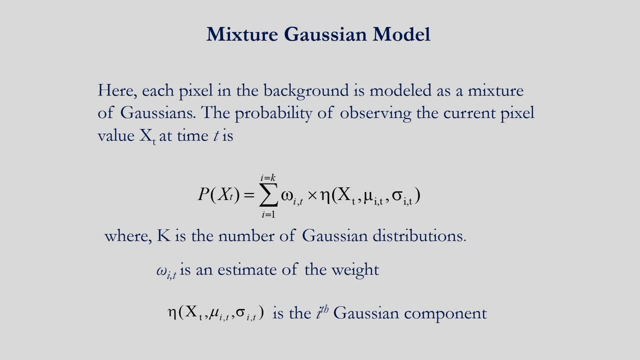 The next one is: I can consider the mixture of Gaussian model that is a mixture Gaussian model. So what is the concept of this? So each pixel in the background is model as a mixture of Gaussians, So i can consider the pixel as a mixer of Gaussian. 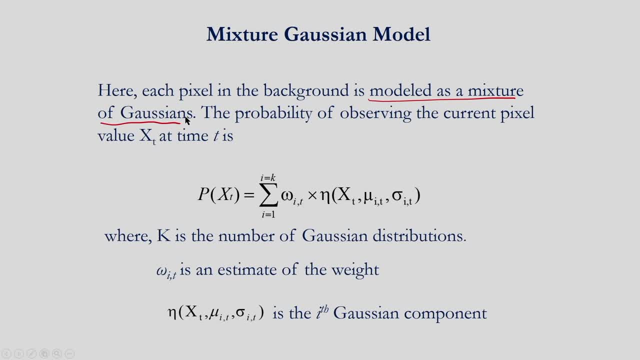 Gaussian model may not be appropriate in many cases. Suppose the background is moving or the maybe the illumination is changing, then in this case the single Gaussian model may not be appropriate. So for this we can consider the mixture of Gaussians And the probability of observing the current pixel value x, t at the time t is given by. 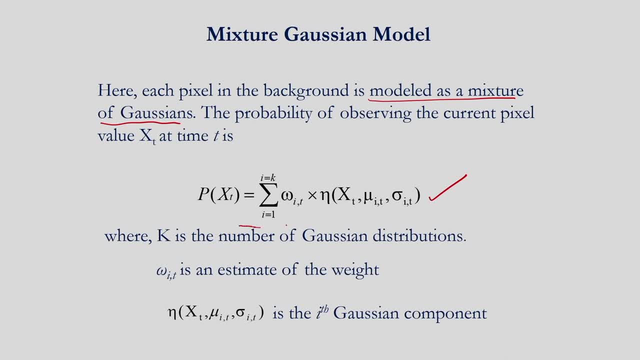 this. So probability of x? t is given by this, And here the k is the number of Gaussian distribution. So how many Gaussian distributions are employed to represent a particular pixel, or maybe the background? And w? i t is an estimate of the weight. So w i t is nothing but the weight. 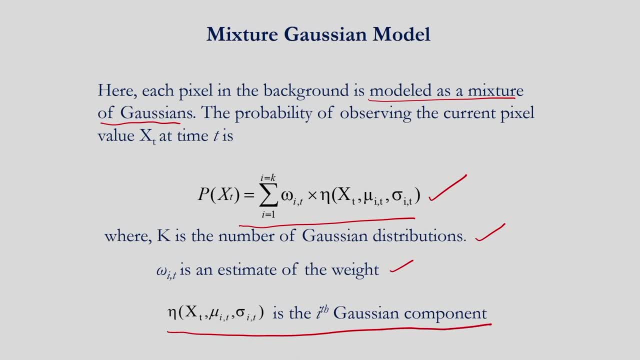 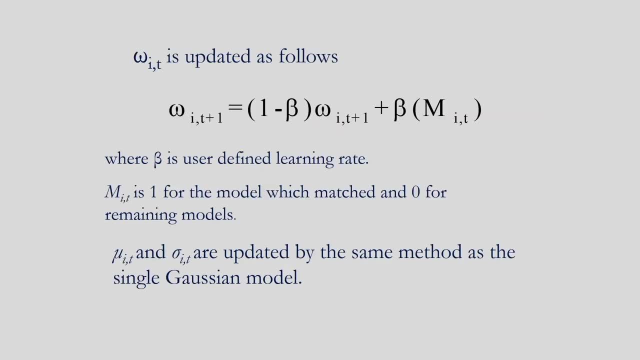 And you can see, I am considering the i, th Gaussian components. So x, t is nothing but the pixel value, and I am considering the mean and the standard deviation. And after this we have to update the weights by using this equation. And here we have to. 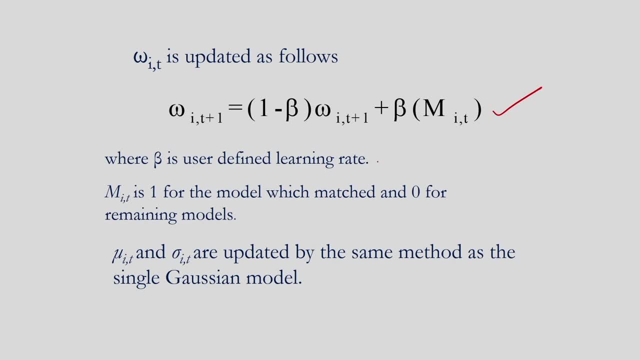 The beta is the user defined parameter, that is nothing but the learning rate, and MIT is one for the model which is maths, and 0 for the remaining models. that is about the MIT And this mean and the mean and the standard deviation, or the mean and the variance should. 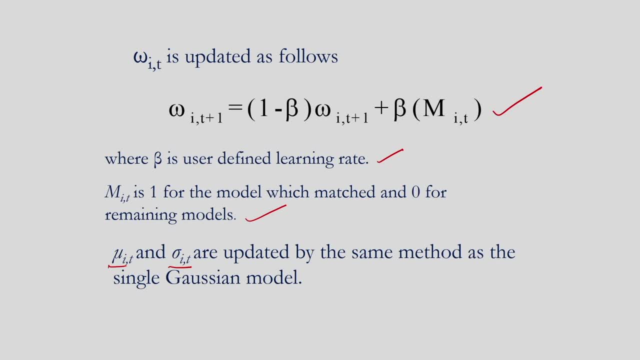 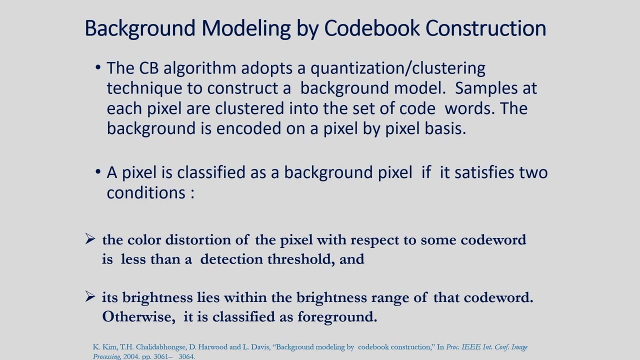 be updated like we did in the single Gaussian model. So this is the concept of the mixture of Gaussian model. So briefly, I have explained this concept, the mixture of Gaussian model, And this is also a very popular method. the background modeling by code, book construction. 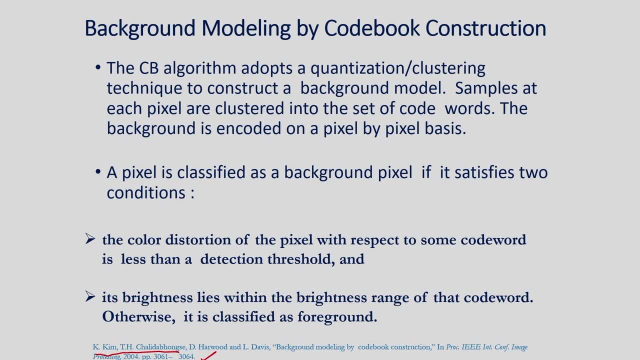 So you can see this research paper by Kim. So this research paper you can see, and I think this is one of the popular method, but this is a very old method now. So in this case, the code book algorithms is employed. that is nothing but the code book. 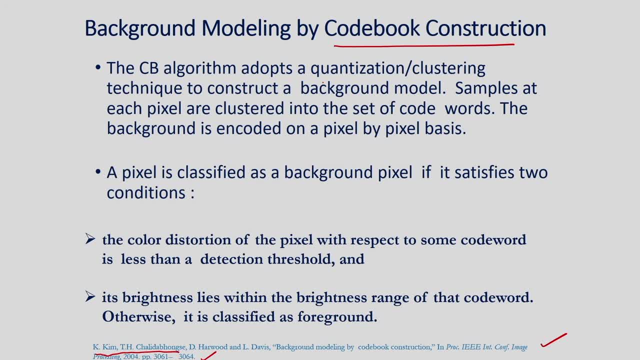 construction and in this case the concept of the quantization or concept of the clustering is employed to construct a background model. So samples at each pixel are clustered into the set of code words, So each pixel that means. if I consider samples of the pixels from the training image, they 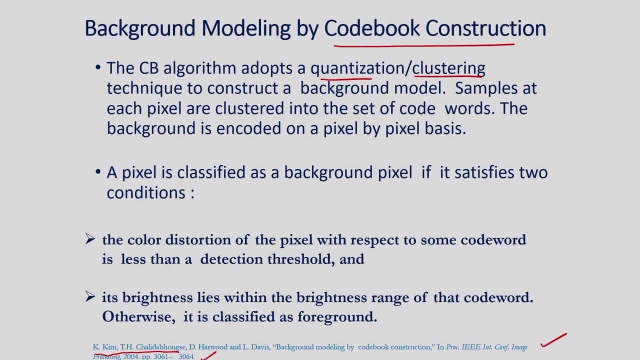 are clustered into the set of code words And the background is encoded on a pixel by pixel basis. So for each pixel, I have the code word and the background is encoded. So the background is encoded on a pixel by pixel basis. A particular pixel can be classified as a background pixel if it satisfied the following: 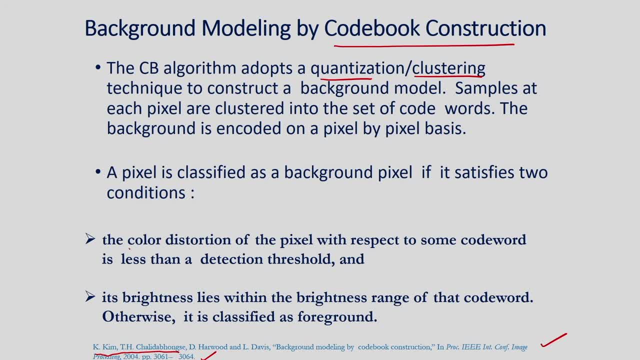 two conditions. So first we have to consider the case of the color distortion. So based on the color distortion we can take a decision whether particular pixel is the, is a foreground pixel or the background pixel. And also we have to consider the brightness difference. 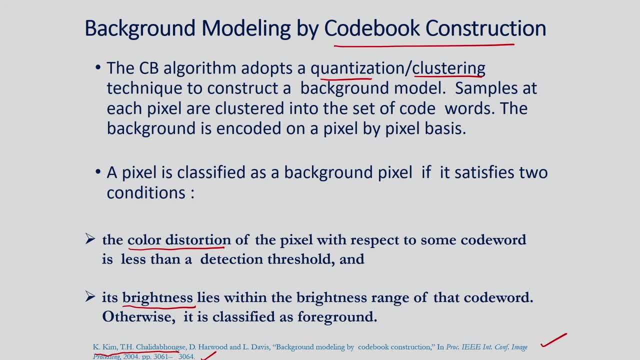 So brightness lies within the brightness range of the code word. That also it is considered And based on this we can select the foreground and the background pixels. So this is the, briefly, the concept of the background modeling by code book construction. For more details you can read this paper. 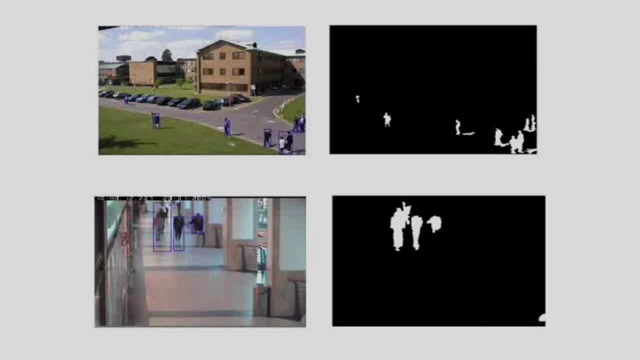 So these are some results. we have done background modeling by the code book technique. So corresponding to this image, you can see I am extracting the foregrounds. And, similarly to this image, I am extracting the foregrounds. Very difficult images in the second image because the background is, you can see, dynamic. 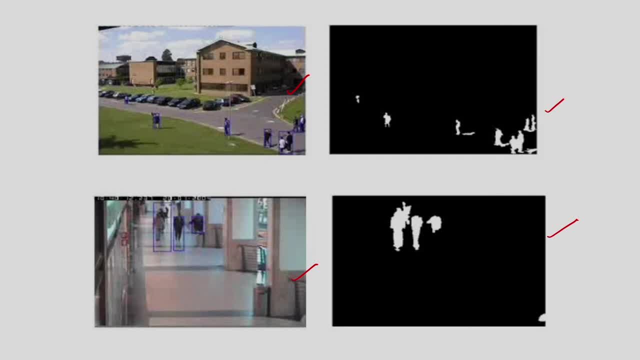 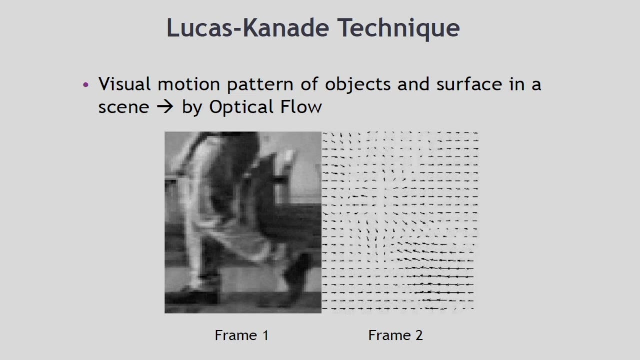 background is also there and also illumination variations are also there and the background is very complex. So these are some results of the background estimation, that is, the foreground, separation from the background, And one important technique is the Lucas Candice technique, that is, the concept of the optical. 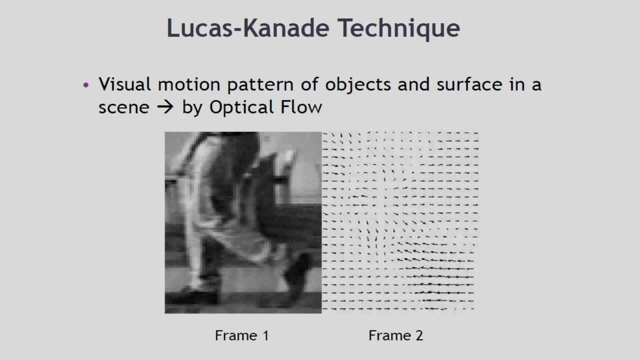 flow, So we can determine the visual motion pattern of the moving objects and that is called the optical flow. So here you can see this person is moving And corresponding to this motion I can determine the visual motion pattern. I can determine, That means I can determine the motion vectors. 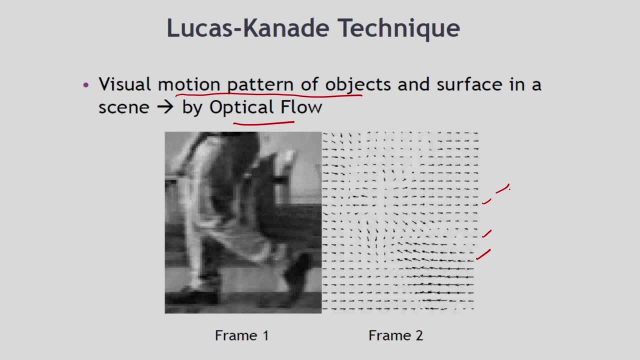 So here you can see, these are the motion vectors. that is nothing but the optical flow. So, based on the optical flow determination I can determine the moving objects. that is nothing but the motion estimation. So this algorithm I am going to explain, That is the motion estimation by optical flow. 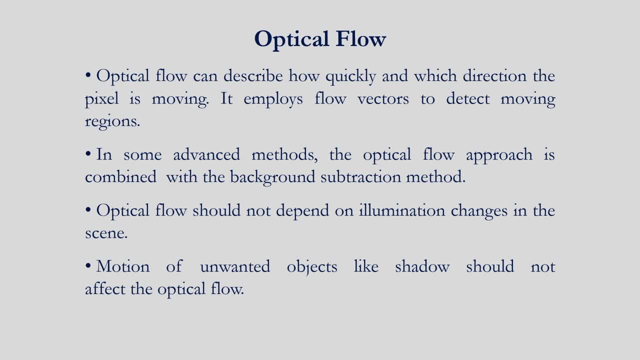 So what is optical flow? This concept is very important. So optical flow can describe how quickly and which direction the pixel is moving. So that means I am determining the motion pattern. That is, the visual motion pattern can be determined by the optical flow algorithm. 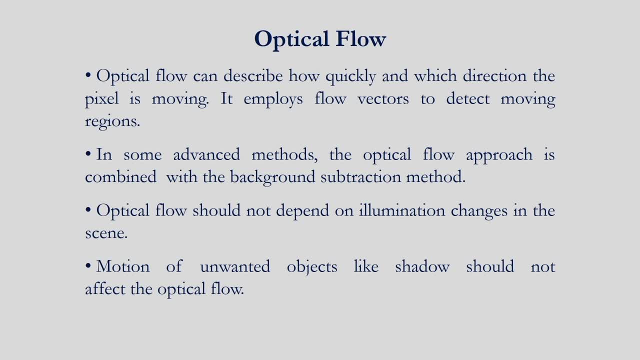 And we can determine the motion vectors- That is, nothing but the flow vectors to detect moving objects, Moving regions. And the optical flow approach can be combined with other background subtraction methods. So by combining this optical flow method and the other background subtraction method, we 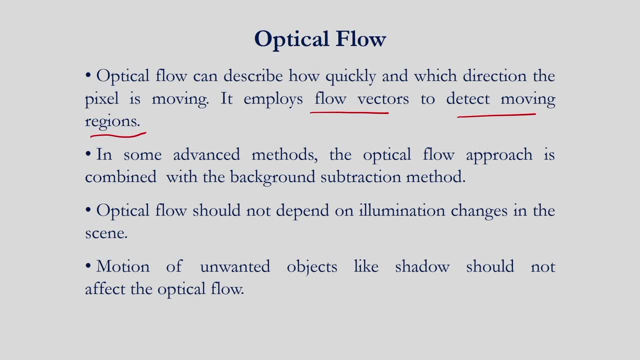 can determine the moving regions. That motion estimation we can do and we can separate the foreground from the background. And I have to consider these assumptions. One is the optical flow should not depend on illumination changes in the scene. That means the illumination should be almost constant for optical flow determination. 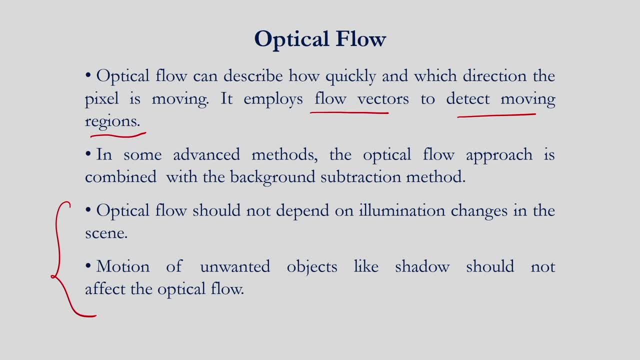 That is one assumption. The second assumption is the motion of the unwanted objects, like shadow, should not affect the optical flow, So that also we have to consider. That means we have to avoid or we should not consider the unwanted objects, And if the shadow is present that will be a big problem for optical flow algorithm. 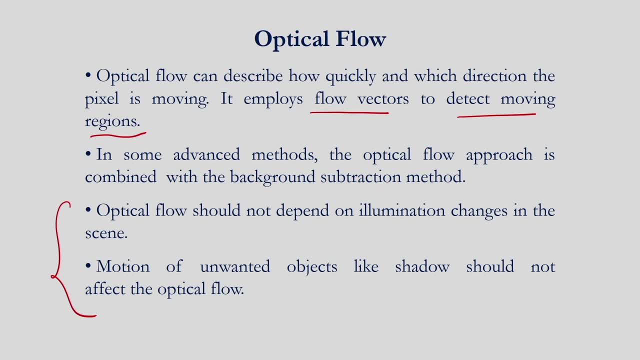 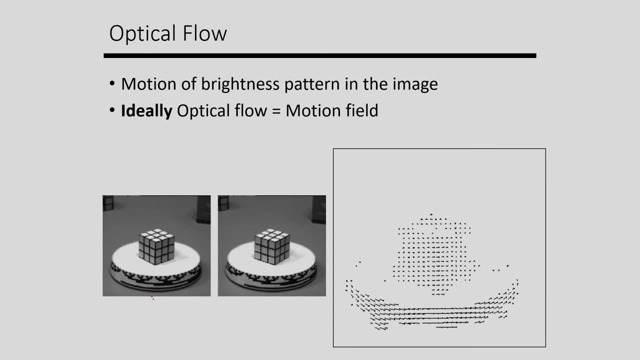 So that we are not considering The presence of the shadow, Or the motion, Or the presence of the unwanted objects. So these two assumptions we are considering for determination of the optical flow. Now let us see how to determine the optical flow. Here you can see in this example I have shown this object is rotating. 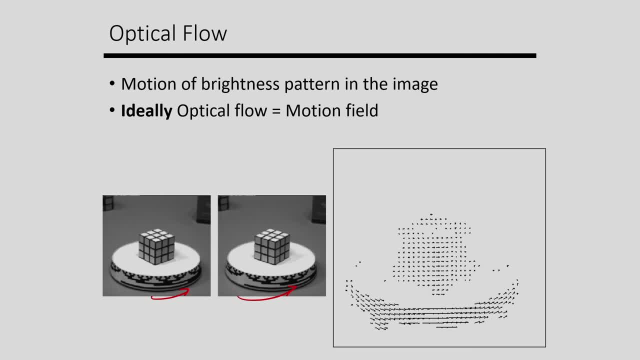 It is rotating like this, in the counterclockwise direction, And corresponding to this, I will be getting the optical flow. That is the motion pattern. I will be getting- And ideally the optical flow is equal to motion field Because the object is also moving. and corresponding to this, I will be getting the motion vectors. 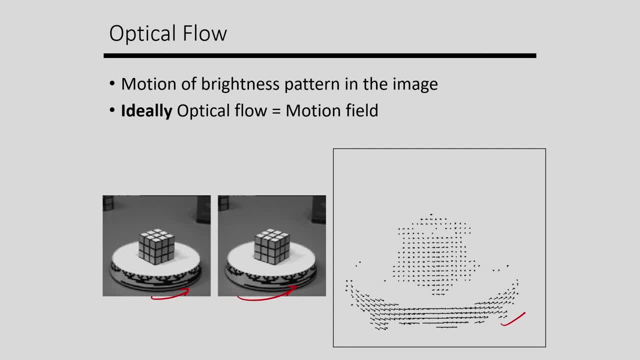 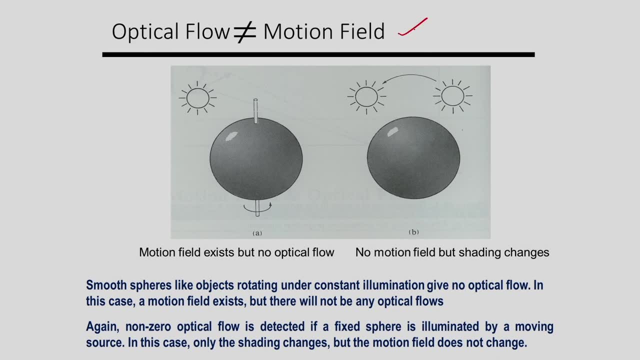 That is the motion field I will be getting And also the optical flow I will be getting. But sometimes it may not be. the optical flow may not be equal to motion field. Here I am giving two examples. In the example A you can see this object is rotating. 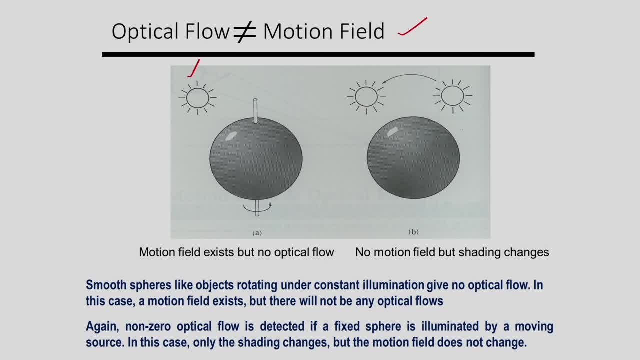 This is rotating And I have the source, One source is available. So corresponding to this path- suppose This path is rotating, That is I am considering- The illumination will be almost constant. That means, if the illumination is constant, then corresponding to this there will not. 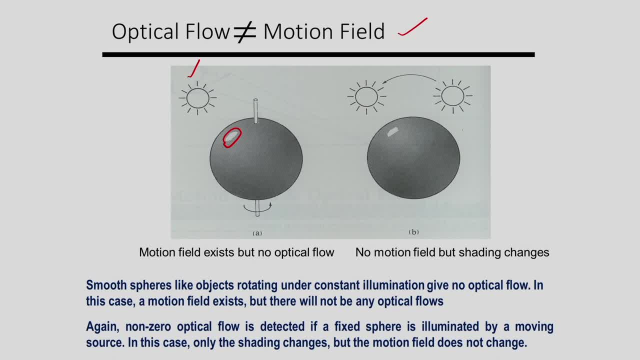 be any optical flow, Because optical flow- how to determine Optical flow- is determined based on the illumination sense, Because the object is moving, and based on this the illumination at different points will be changing, But in this case the illumination at this particular point, it will be almost constant. 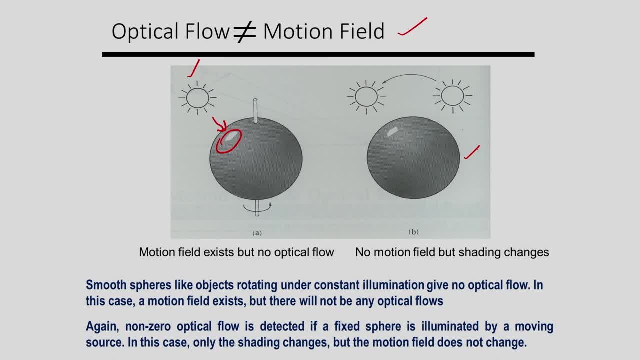 There is no motion. you can see, The object is in stationary, that is, the sphere is in the stationary. But I have the moving sources. The source is moving, So corresponding to this path, suppose I have different brightness, The brightness will be changing. 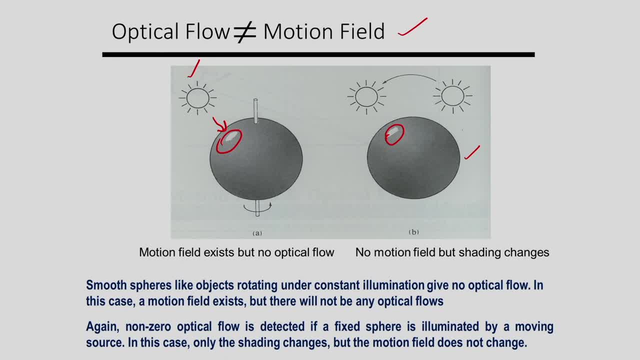 So whenever the brightness is changing, the, I will be getting the optical flow, But I will not be getting the motion because there is no motion field here. The motion field is zero. So Instead of having the motion is zero, the optical flow is present. 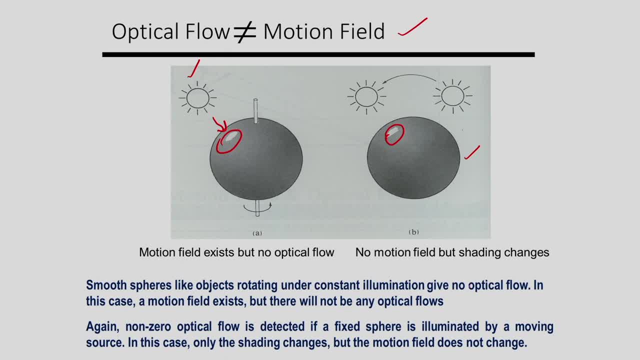 So that means no motion field but shading changes. That means the brightness corresponding to that particular paths. it will be changing because the sources are moving. So in the first case, motion field is there but there is no optical flow. In the second case, motion field is not there but there is a change of the brightness and 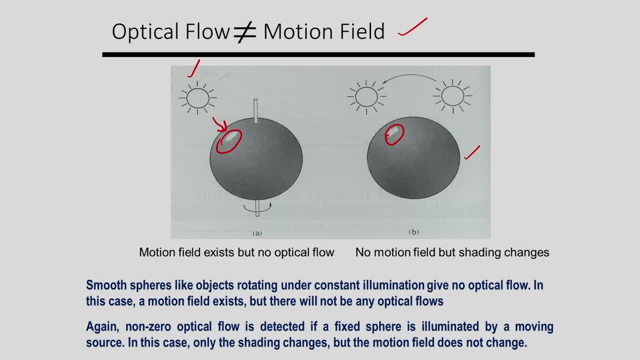 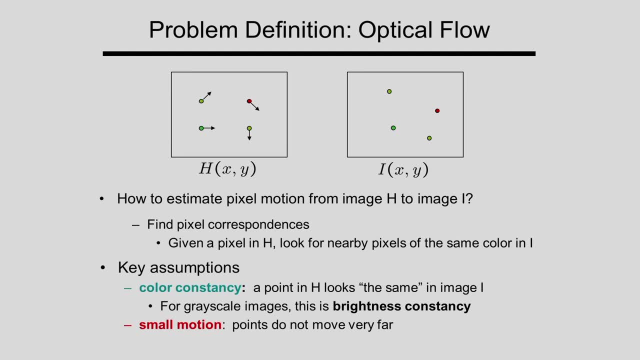 because of this. So I will be getting the optical flow. So that means I can say the optical flow is not equal to motion field. And the problem definition of the optical flow. So here I have shown two images, one is H, another one is I. 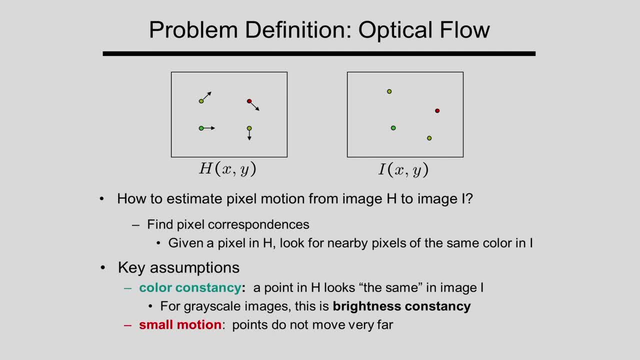 And I have shown some pixels, the red pixels, the green pixels, like this I have shown, And the pixels are moving. So I have to determine the motion of the pixels. That is nothing but the motion estimation. So for this, You can see, 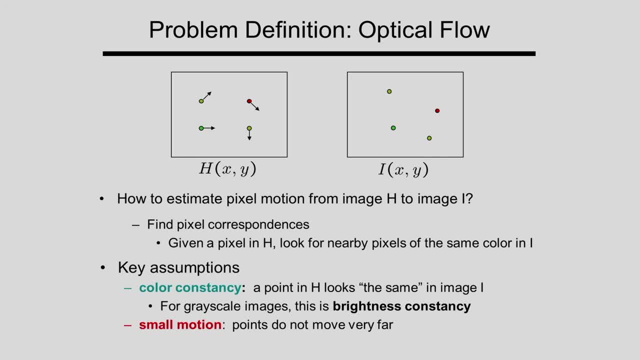 Find the pixel correspondence. So I have to find the correspondence between the pixels And based on this I can determine the optical flow, I can determine the motions. So suppose this red pixel is corresponding to this red pixel And similarly this pixel is corresponding to this pixel, like this: 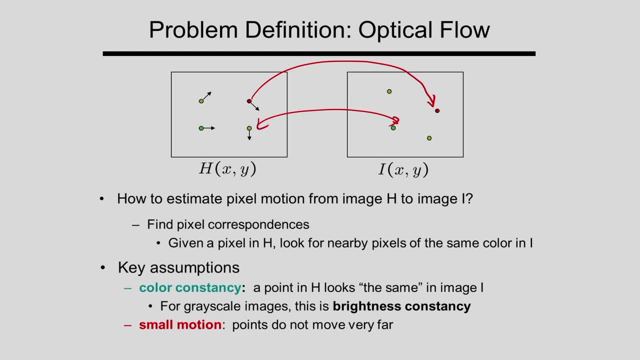 So I have, so I have to find the correspondence between the pixels. So for this I can consider some assumptions, like the color property I have to consider, or maybe the brightness property we can consider For the gradient, For the grayscale image, And also we have to consider this assumption, that is, the small motion assumption we have. 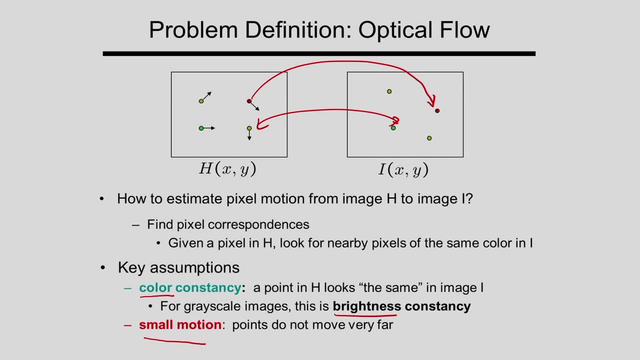 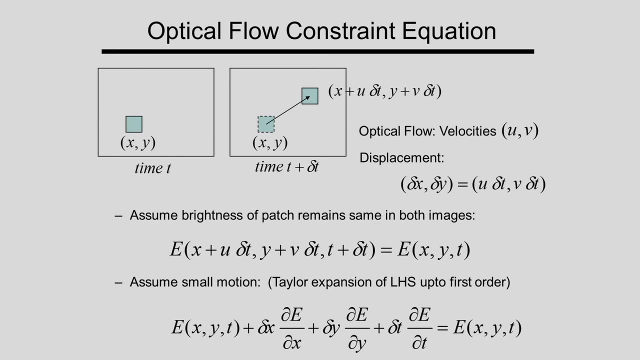 to consider Points do not move very far. So for this I have to find the correspondence between the pixels of the images. So the actual concept of the optical flow I will be explaining in the next slide. Here I have shown two frames of a video at time t. another one is time t plus delta t. 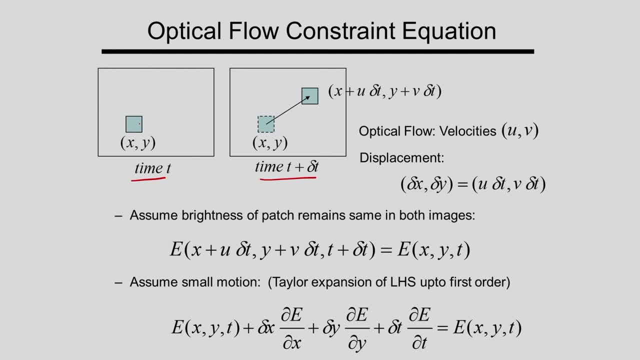 And let us consider a patch at the point x, y. So this patch I am considering, And at the time t plus delta t, this patch moves to the this position, the second position, So this patch will be moving. suppose Now what will be the position of the patch in the second image. 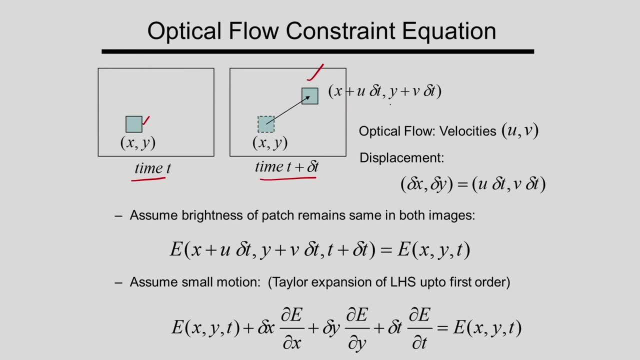 The position of the patch in the second image will be x plus u delta t, comma y plus v delta t. So in this case, what is x plus u delta t? u delta t is nothing but delta x. So that means It is nothing but delta x. 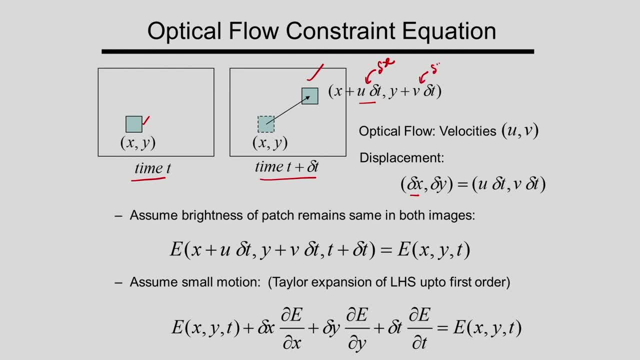 And similarly the v delta t. it is nothing but the delta y. So what will be the position of the patch in the second frame? The position of the patch in the second frame will be x plus delta x comma, y plus delta y, And I am considering the velocity, that is, the optical flow velocities u and v. 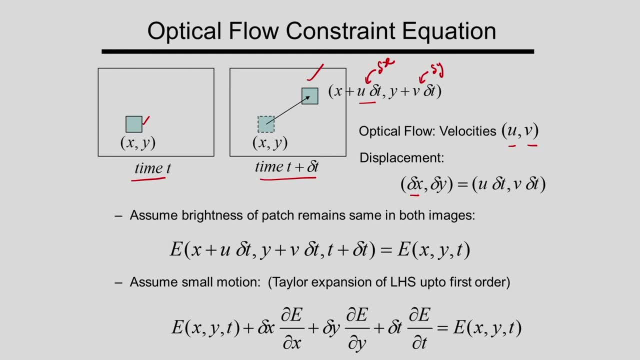 So u is the velocity along the x direction and v is the velocity along the y direction. So from u and v I can determine the displacement. So delta x is nothing but u delta t and delta y is nothing but v delta t that I can determine. 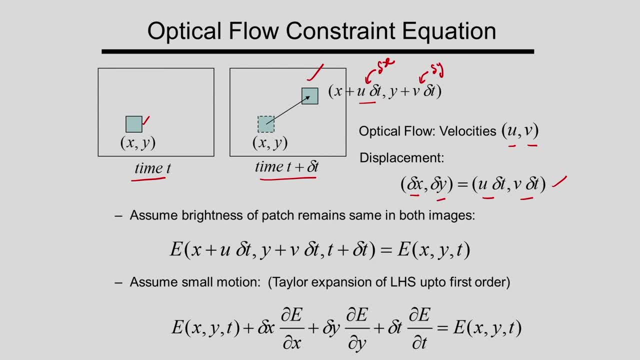 So assume that the brightness of a patch remains same in both the images. That is true. here you can see this patch is moving to the moving to this position, the second position. So that means the brightness of this patch will remain same in both the images. 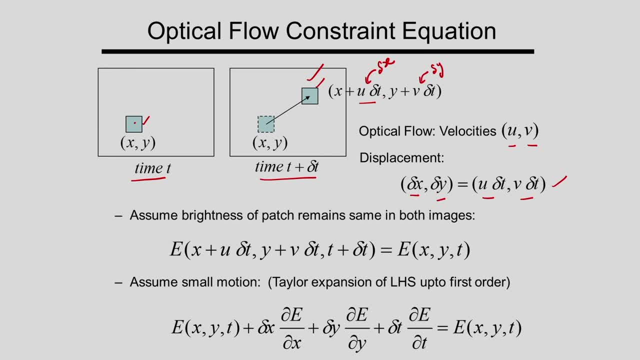 Only the position is changing, but the brightness of the patch remains the same in both the images. So here you can see: that is the brightness at the point x comma y at the time t. So e is the brightness of the patch at the point x comma y and at the time the time is: 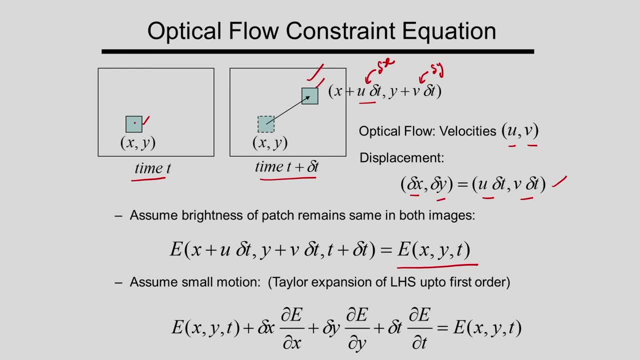 t, and since the patch is moving to the another position in the time, t plus delta t, the same patch is moving, So there will not be any brightness since. So, corresponding to this, what will be the? what will be the brightness? The brightness will be e x plus u delta t, because that is the new position: x plus delta. 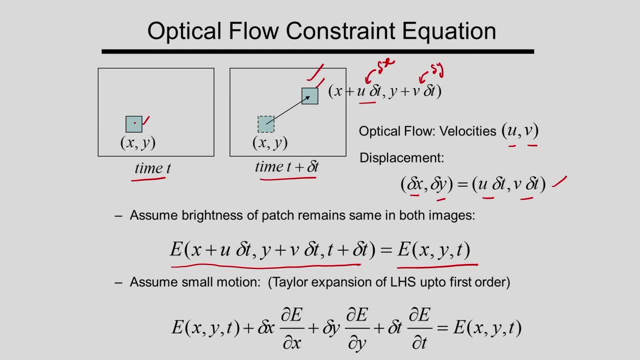 x comma y plus delta y, and what is the time? the time is t plus delta t, So brightness will remain same. So I can show another diagram. suppose suppose I am considering one object and it is rotating. suppose So this object is rotating like this, so this is at time t and this is at t plus delta. 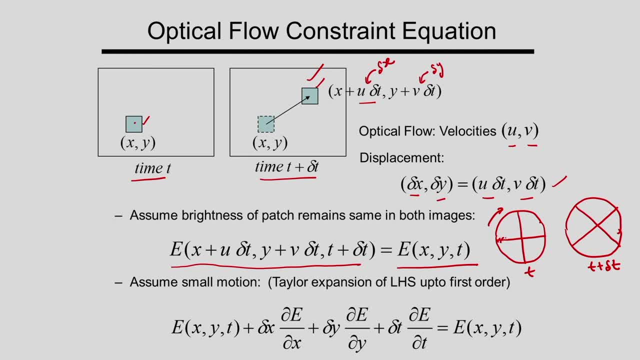 t. So if I consider the brightness at this point, suppose will be same as that of this, because this point is moving and this is moving to this point, So brightness of this will be same. So if I consider the same position, so brightness at this position- the position number 1- and 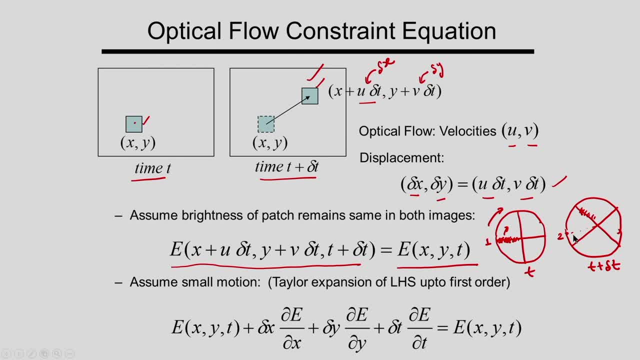 the position number. suppose the 2 the same position. it will be changing because of the rotation. So from this I can determine the optical flow here you can see corresponding to the position 1 at the time t and corresponding to the position 2 at the time t plus delta. 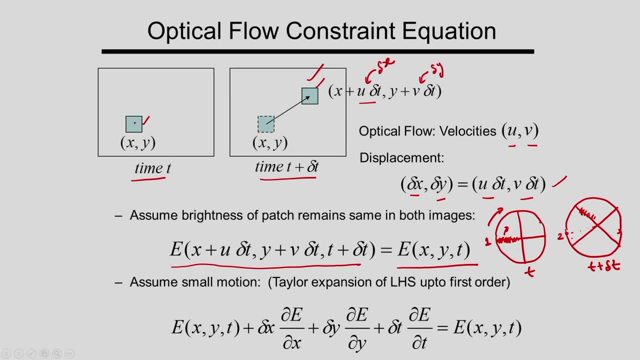 t, the brightness will be different because of the rotation. So, based on this concept, I can determine the optical flow, because the brightness at the same point, because this point and this point is the same point 1 and 2 is the same point. 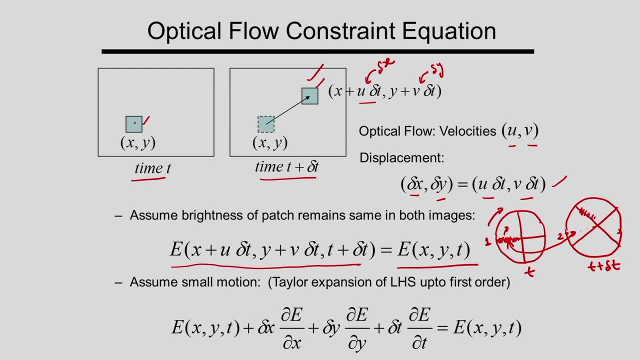 So brightness will be different because of the rotation, So that gives the optical flow. So now you can see the assume brightness of the paths remain same in both the images. then I will be getting this equation and this I can expand by considering the Taylor series. 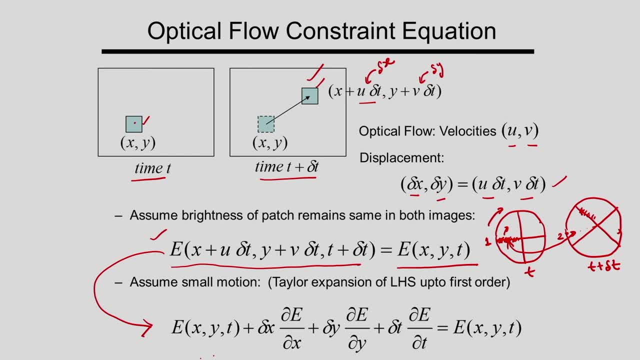 expansion, So higher order terms. I am neglecting, So I will be getting this one. So this equation: I will be getting and I can cancel out this, this and this will be cancel out. So from this what I will be getting. 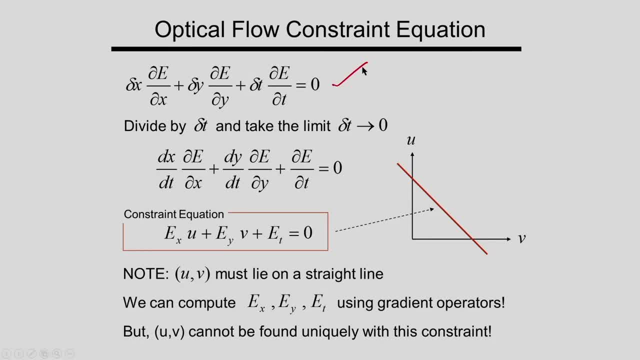 So I will be getting this equation, delta x, delta e divided by delta x plus delta y, into delta e divided by delta y plus delta t. delta e divided by delta t is equal to 0 and divide by delta t and takes the limit, delta tends to 0. 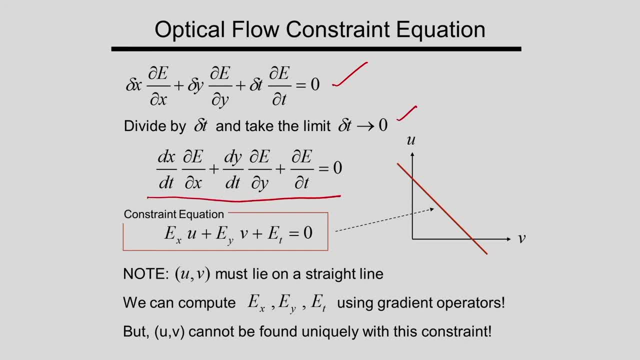 So from this I will be getting this equation. So I have to divide by delta t, So I will be getting this equation. and this equation can be represented like this: So I will be getting this one, the E x u plus E y v plus. 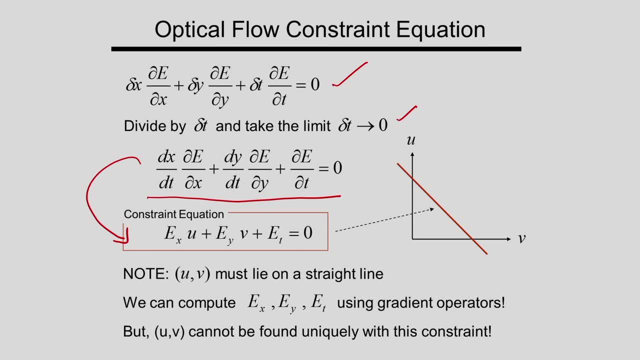 E, t is equal to 0. So what is E x? What is E x in this case? E x is nothing but delta e divided by delta x. that is the change of brightness with respect to the coordinate. the coordinate is x, that is the special change of the brightness. And similarly, if I consider 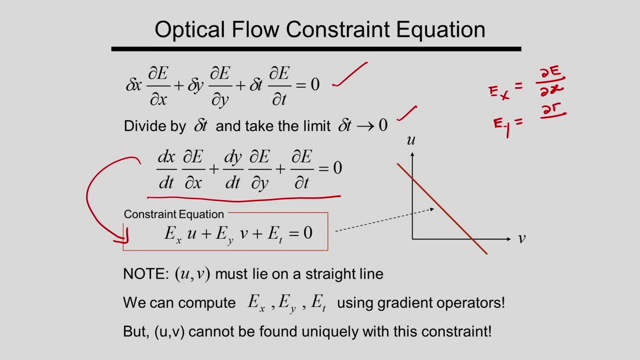 E, y, that is nothing but delta e divided by delta y. This corresponds to the special change of the brightness because of the motion. And what is the d x d t? d x d t is nothing but u, that is, the velocity along the x direction. and what is the d y d t? So d y d t is nothing. 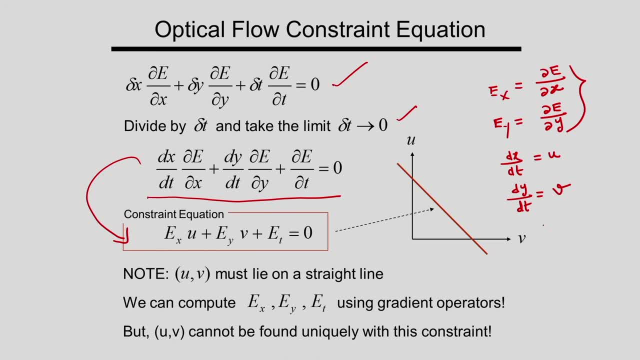 but velocity along the x direction, the y direction, that is v. and what is delta e, delta t, that is the time rate of change of brightness. The brightness is changing with respect to time because already I have explained, suppose this object is moving like this at time t and at the time t plus delta. 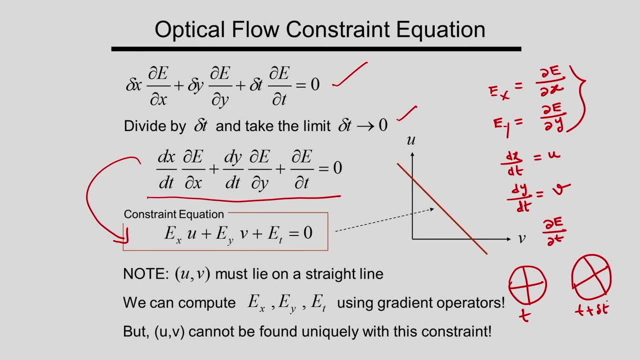 t. So this is a t plus delta t. So you can see the brightness at this point. So brightness at this point, suppose 1 and 1, it will be changing. So change of the brightness with respect to time. So that is delta e divided by delta t. So I will be getting this equation. 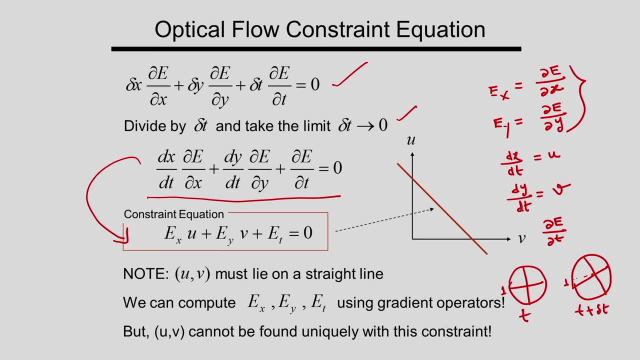 This is the equation of a straight line, So the velocity u and v must lie on a straight line and based on this we can compute e, x, u, y and e, t using the gradient operators. But the problem is- it is not a simple problem- u and v cannot be found uniquely. What we 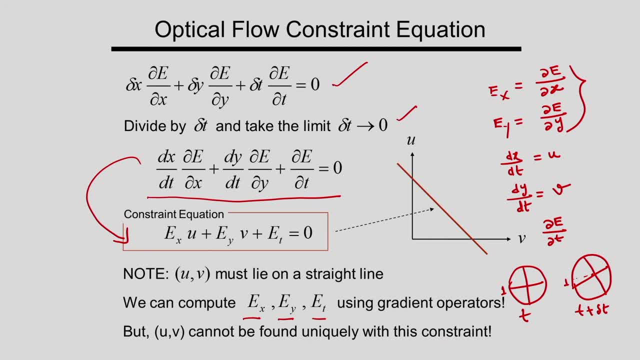 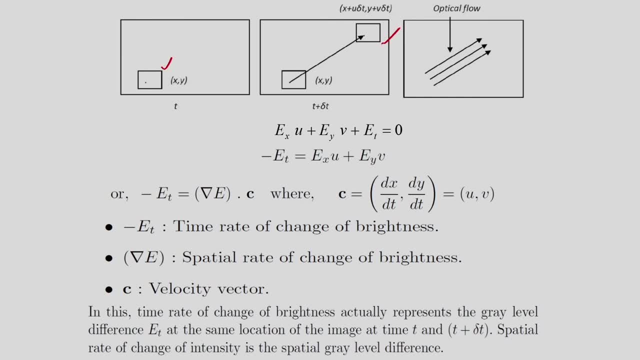 can do is with this constraint. So with this constraint I cannot determine the velocity u and v. So the same concept I am showing here, So this path, it is moving to the, this position and corresponding to this, I will be getting the optical flow, The optical flow. 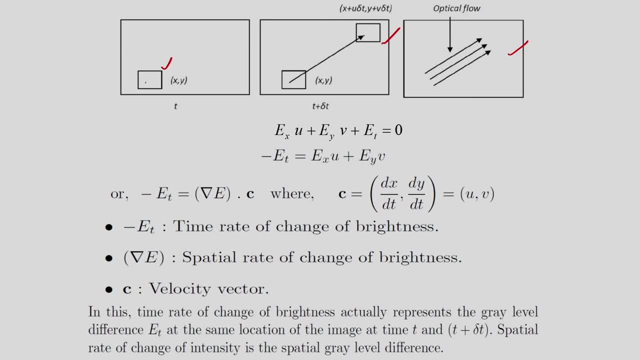 it depends on the change of the brightness because of the motion. So already I have this equation. So this equation I can write like this: So what is the interpretation of this equation? You can see, I will be getting this equation from this: minus e, t is equal to that is the delta e. 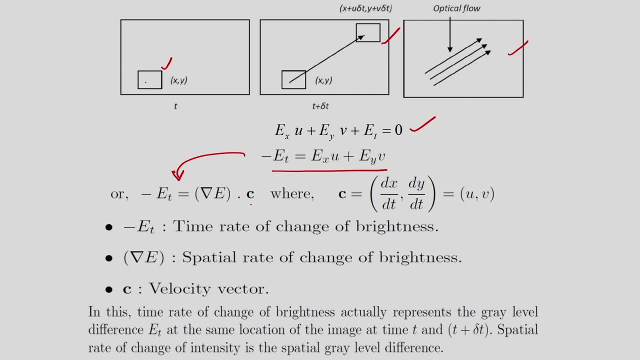 that is the gradient of e, dot c. So c is nothing but the velocity vector. So c is the velocity vector. So I have two components: One is the u, another one is the v Velocity along the x direction and the velocity along the y direction. And what is e t? e? t means? 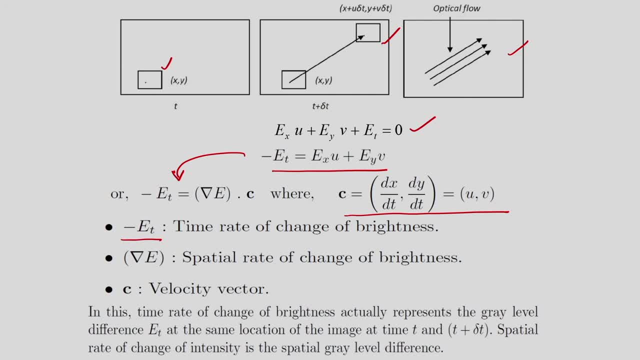 the time rate of change of brightness. So, with respect to time, the brightness will be changing Because of the motion. That is the time rate of change of brightness. And what is this? delta e? Delta e is nothing but the spatial rate of change of brightness. So one is the. 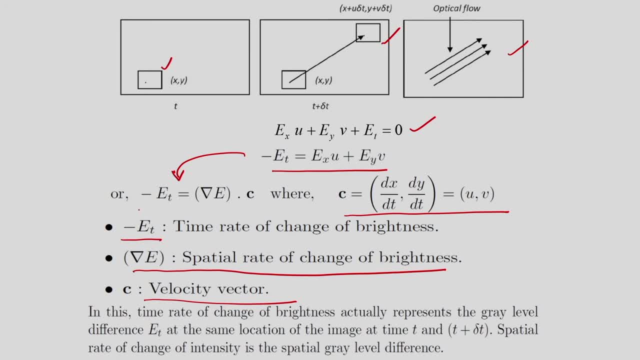 velocity vector. So our objective is to determine the velocity vector from this equation. So this is the equation, This is the constraint equation, or the optical flow equation. So from this equation we can determine the velocity vector. The velocity vector is c, So c is. 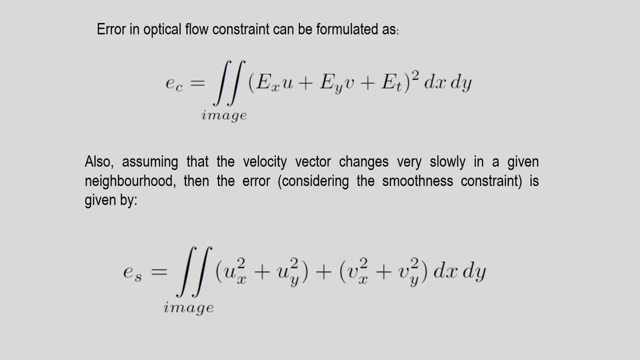 So I have two components, u and v, And for optical flow solution there are many methods, So simply I am showing one method, but if you want to see the solution of this method so you can see the optical flow paper. research paper by Horne. the original paper is by Horne. 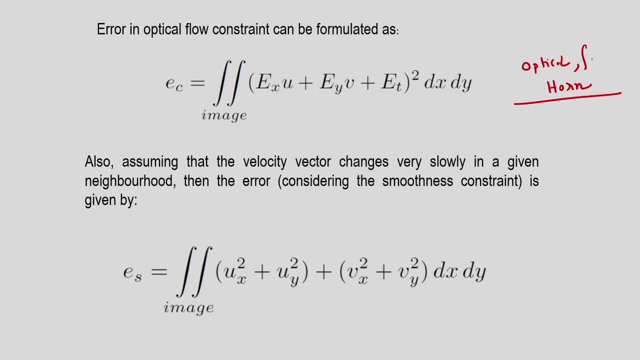 so you can see this research paper, the optical flow, optical flow algorithm. you can see by Horne. but briefly, I have explained the solution of this equation and that is the optical flow equation. So for this we have to consider error in optical flow constraint. 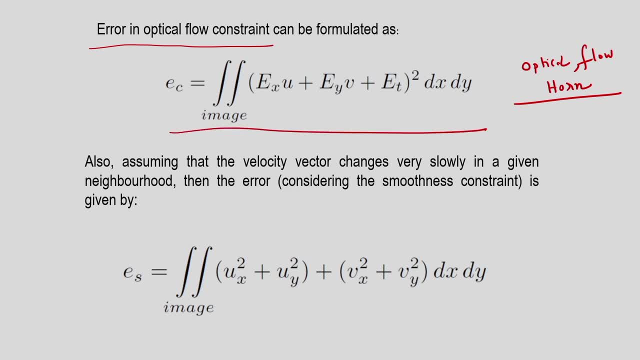 So this error I am considering and also we have to consider another assumption, that is, the velocity vector changes very slowly in a given neighborhood. that means the motion is very slow. So this assumption I have to consider, that is nothing but the smoothness constraint we 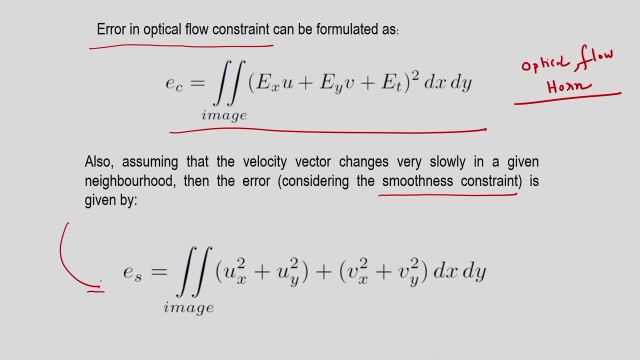 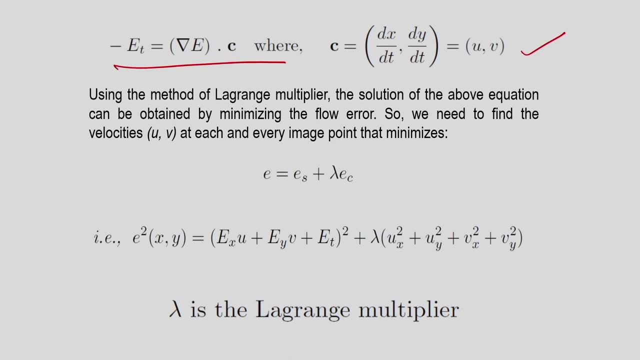 have to consider And based on this I am having this equation. that is nothing but the smoothness constraint. So already you have this equation, that is the optical flow equation, and this equation we can solve by considering the Lagrangian multiplier method. 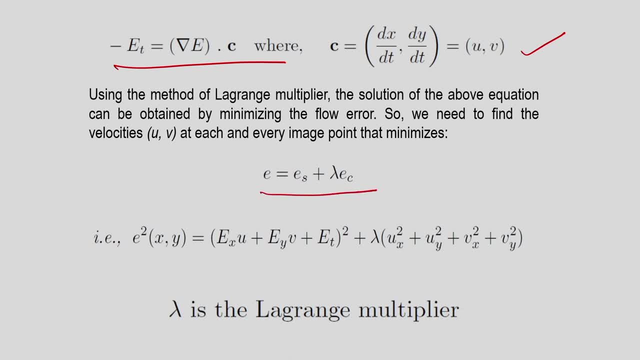 So E is equal to E s plus lambda E c that we can consider. So lambda is nothing, but it is the Lagrangian multiplier And based on this error, the flow error, already we have calculated. So E is equal to E s plus lambda E c. we have already defined E s and also we have 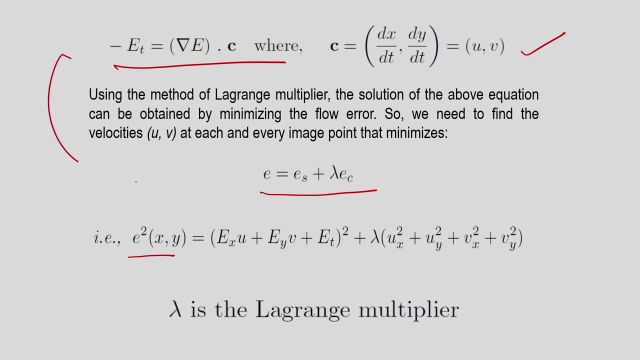 defined E, c. The solution of this equation we are considering like this: we have to minimize the error and we will be getting this one. So we have to do some mathematics and I will be getting this one. And after this, the solution of this equation is nothing, but I will be. I have to do the 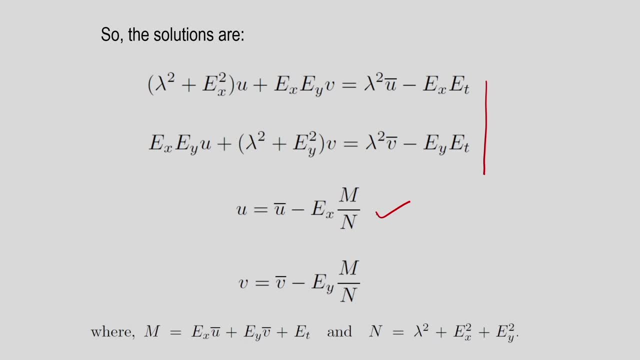 solutions. And finally I will be getting the velocity along the x direction, that is, the u I can determine, and velocity along the y direction I have to determine. u bar is nothing but the mean velocity. these are the mean velocity and m is defined like this: m and n is defined like this: 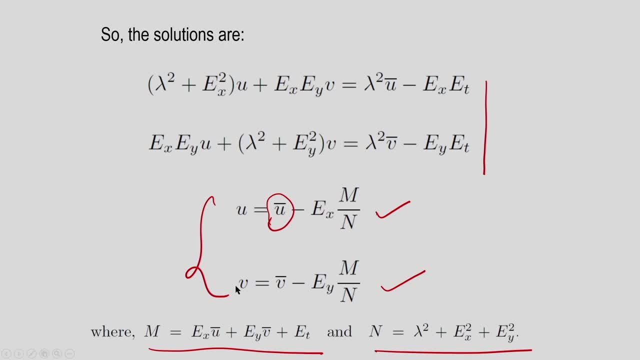 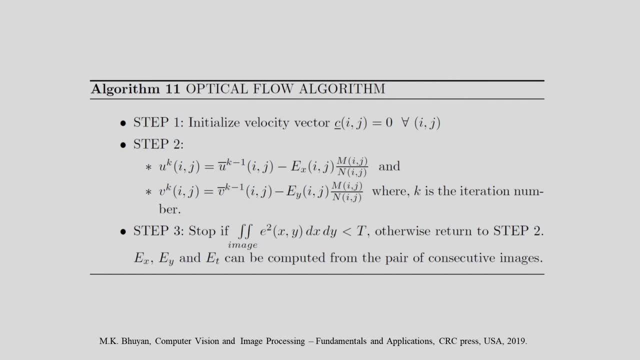 So from these two equations I can determine u and v. that is the velocity vector I can determine. So I can show the simple algorithm from my book, optical flow algorithm. So initialize velocity vector. first I have to initialize the velocity vector. 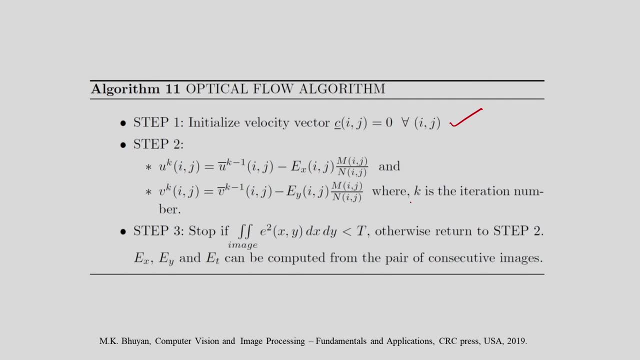 After this I have to consider the iterations, So k number of iterations I am considering. So by using the previous equations you can see I am calculating the value u and the v and we have to stop these iterations. So first we have to consider this error. the error should be less than a particular 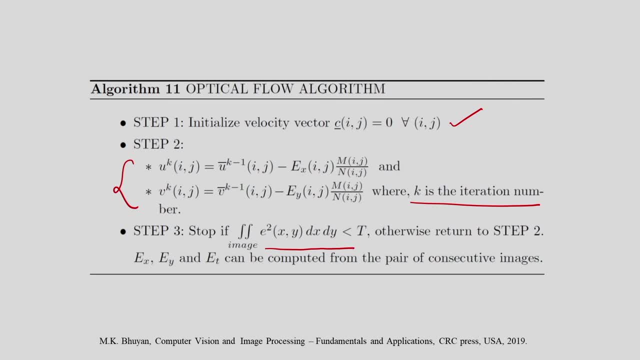 threshold and based on this we can stop the iterations. Otherwise I can I have to continue the iteration and I can determine the u and v. So this algorithm I can employ in a video. So in a video I can use this algorithm. 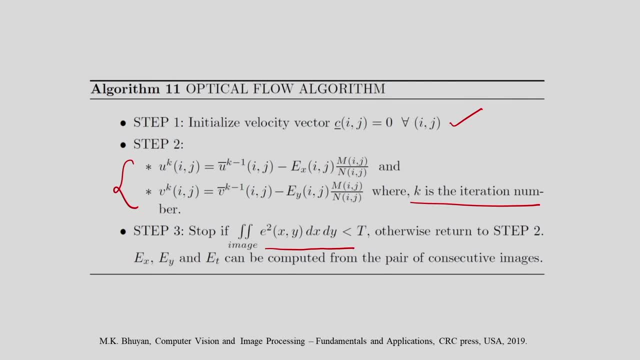 So in a video I can use this algorithm. So in a video I can use this algorithm. So in a video I have the frames, number of frames. So in that case the k is the frame numbers. 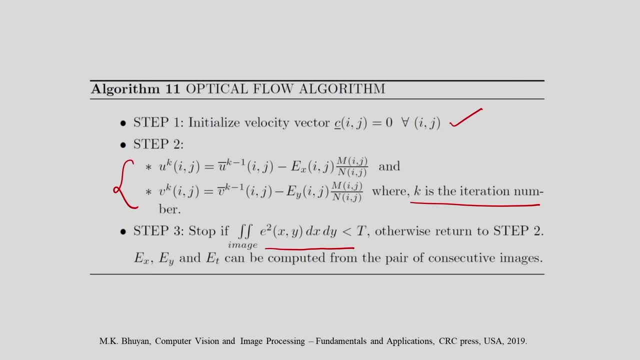 So all the frames I have to read one by one, one number frame 1, number frame 2, like this. So k number of frames of a video I have to read and from this I can determine the velocity along the X direction and the velocity along the Y direction.